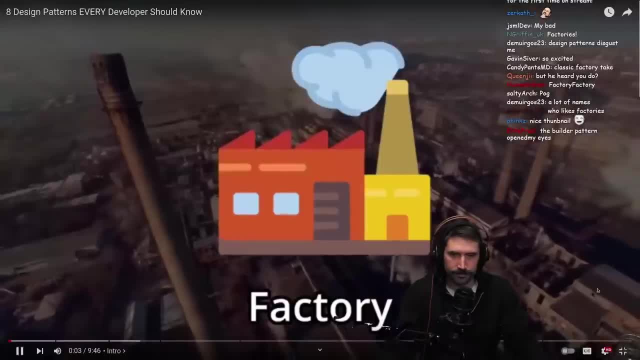 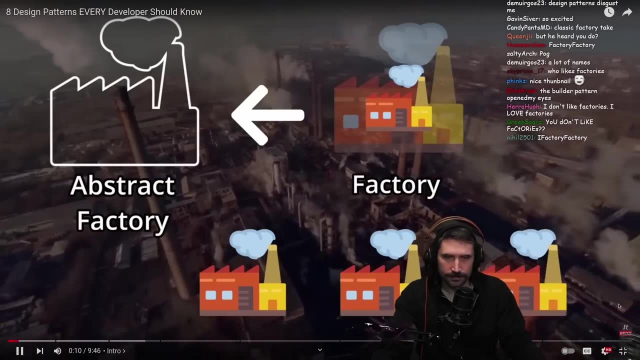 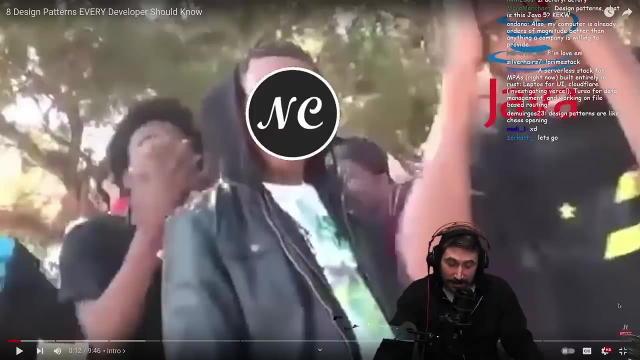 I heard you liked factories, so I made you a factory inside a factory which inherits from an abstract factory, so it can create new factories. But enough about programming in Java. You know, I mean at Netflix on the originals team. Okay, so in 2017, when originals were really 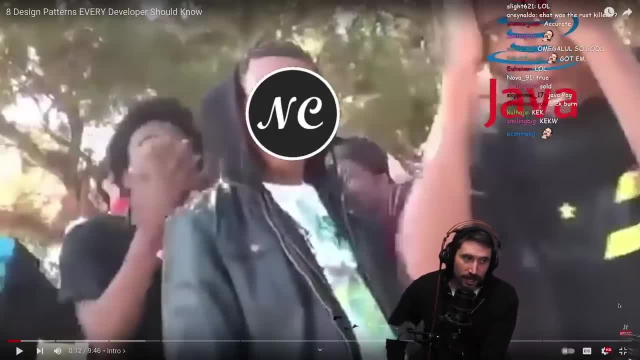 getting started real talk. we did have an abstract. We had an abstract builder factory. Okay, it was an abstract builder factories that would produce images and other assets for all of our new original content. So I mean, I did have, I did get the full abstract builder factory. 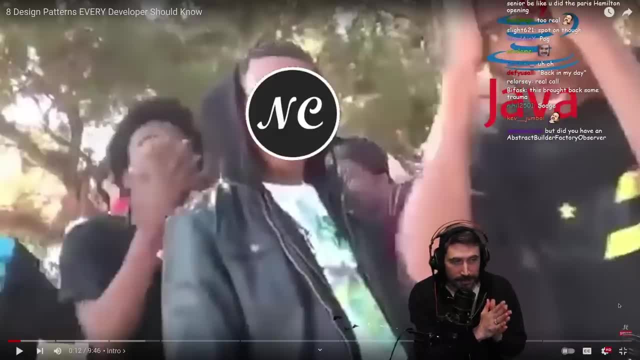 right, Like I think that's really a winner. If I'm not mistaken, we also we had an abstract factory. We also had the abstract factory factory. We had, like we had it all. We had the builder config factory. for sure that you'd build up a config. 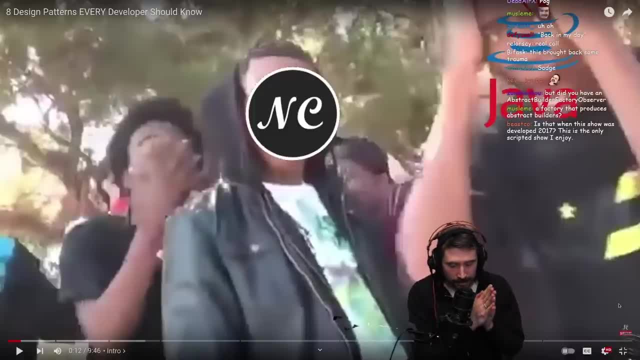 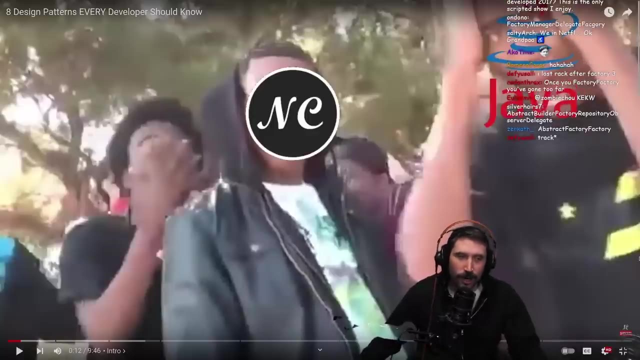 and then you'd produce it And it was super complicated And I got most of it down. But man, those days in Java, you know, Java, Java is a lot, of, lot, of, lot, lot of factories. You know what I mean. You just get fucked up, right. It's just like if you ever want a good factory, 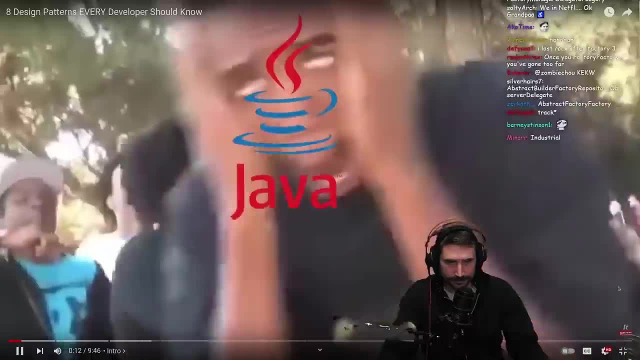 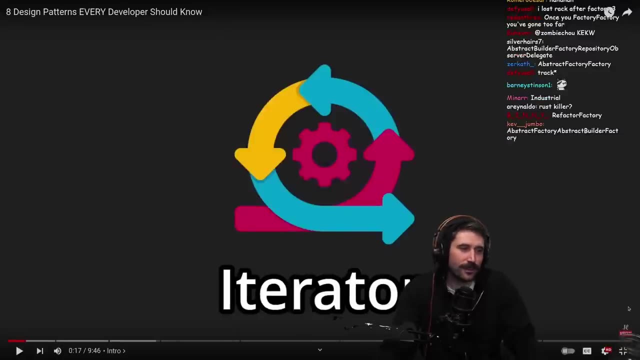 factory. go get it, get it. in this video we will learn about eight design patterns. every developer should. strategy is the only the strategy pattern. strategy pattern is like the greatest pattern of all time. okay, everyone uses the strategy pattern. uh, second off iterator pattern. real good, no, in 1994 the gang of 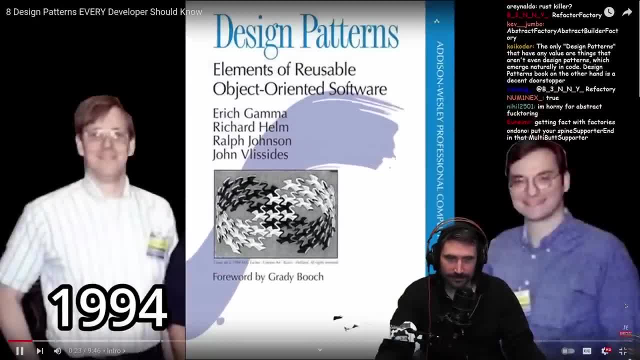 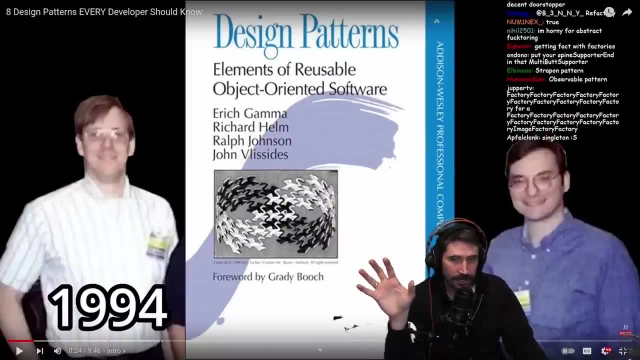 four released the holy book design patterns, introducing 23 object. by the way, if you haven't read this, you should, even if you don't like. oop this. this idea of patterns that can exist within software is really amazing, and it also works in things like rust. there is patterns in rust being 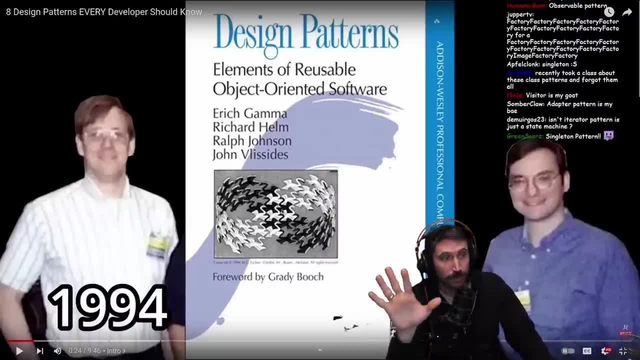 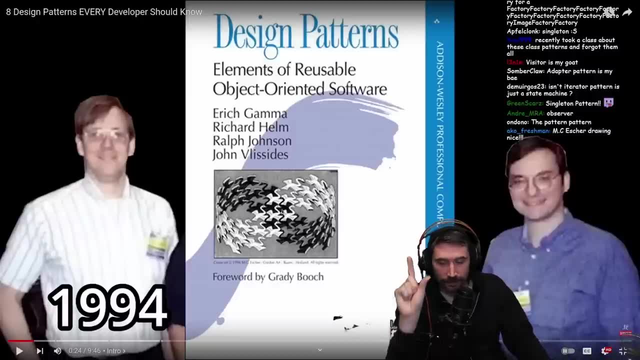 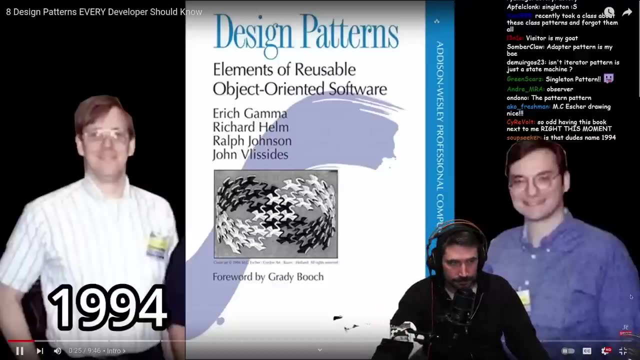 able to understand patterns and like abstract them out and reuse a strategy to write software. i think is one of the best things you can do, because no matter what software you write, there are patterns that can make things simpler and make other people get up to speed. oriented design patterns. 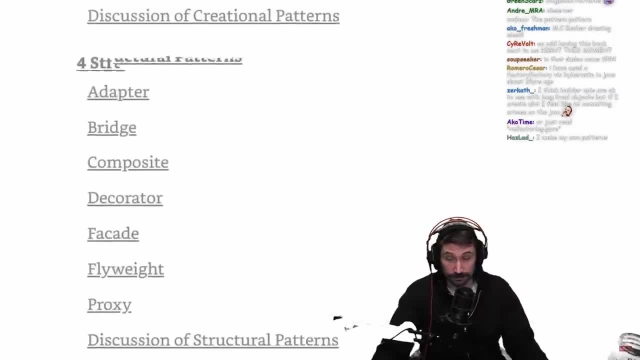 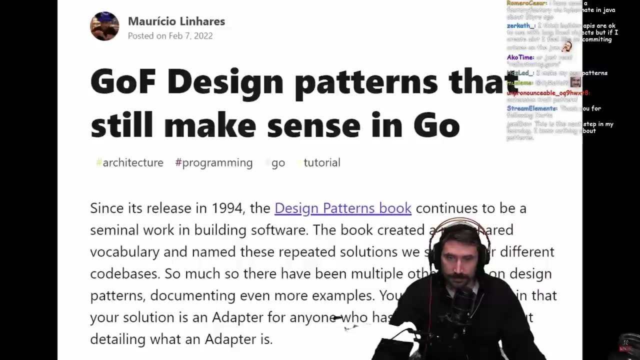 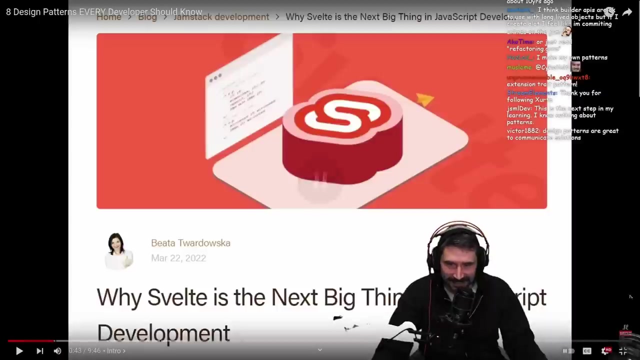 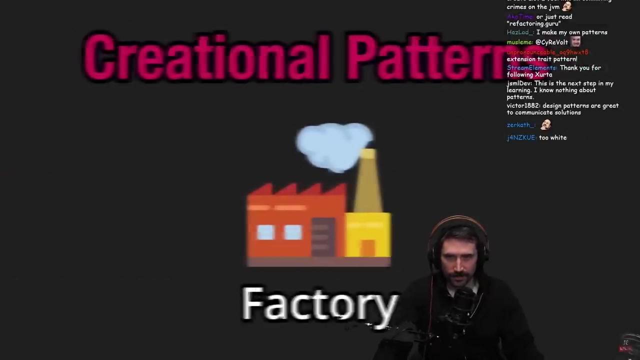 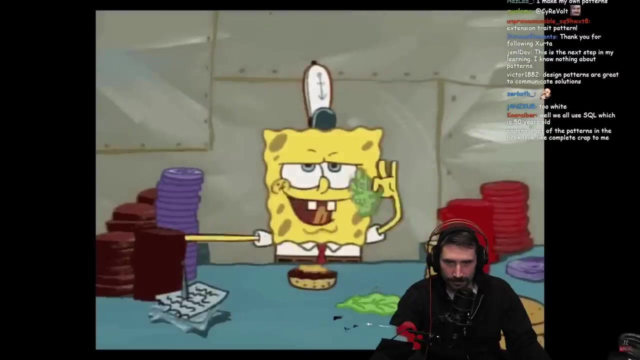 so let's just. let's just be real here. if only, if only react was dying. okay anyway, style faster than you can say javascript was a mistake. anyways, let's start with our first creational pattern: the factory. imagine that you want a burger but you don't want to have to worry about getting all the ingredients and putting them. 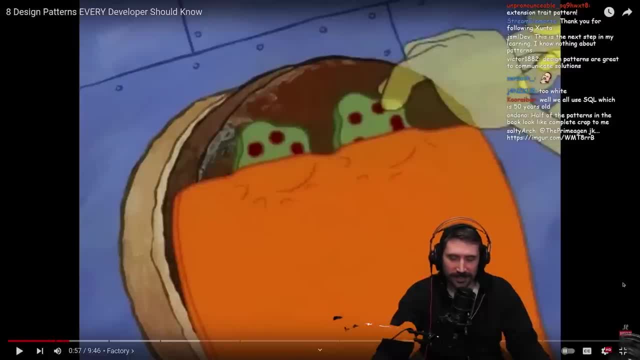 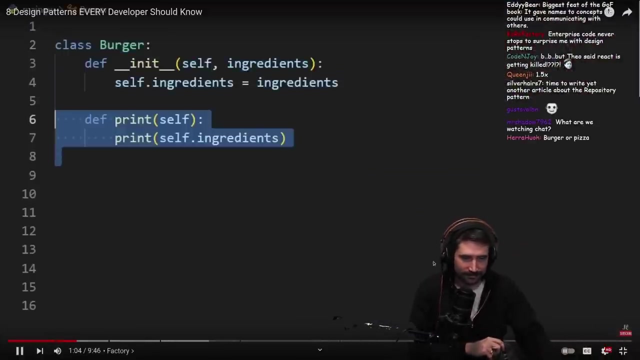 together. you know, this is always how this, this pattern, is des described. i always feel like it starts. it's verbally so simple, but it's always a huge pay in the ass anyways, so instead you just order a burger. well, we can do the same thing with code, if it takes a list of ingredients to create a 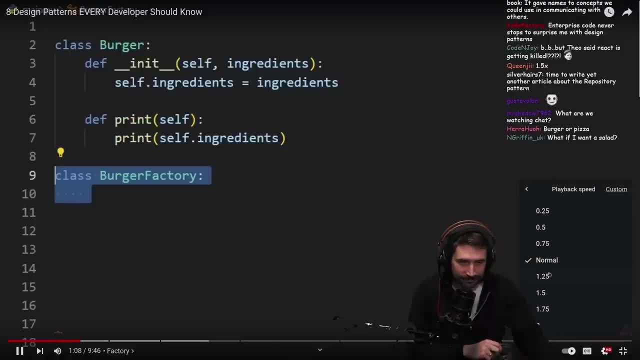 burger. we can instead use aging. how god the sater house you a dreaming who that was said to be a? We can instead use a factory which will instantiate the burger for us and return it to us, whether it's a cheeseburger, a deluxe cheeseburger or even a vegan burger. 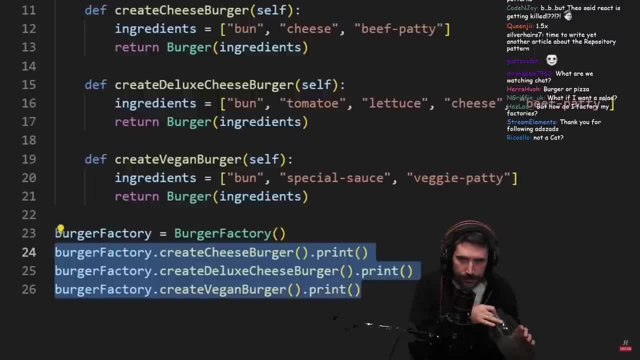 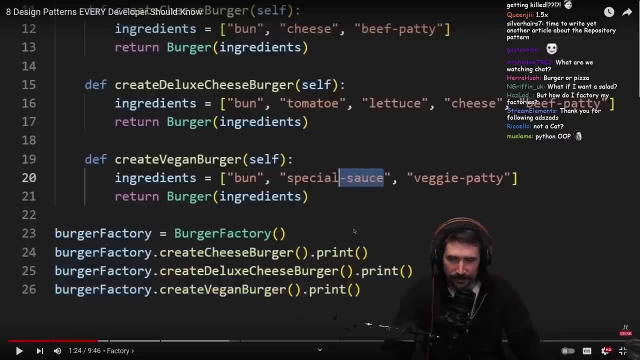 All we have to do is tell the factory what kind of burger we want, just like you would do at a restaurant. But be careful, because this way you'll never- Again. you know this always is the- I mean. like when you look at this for a second you. 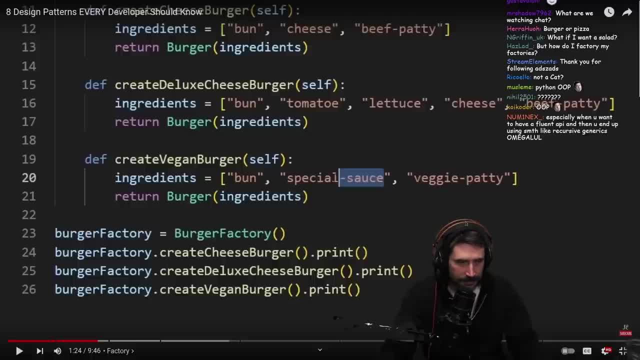 realize, like how annoyingly coupled this is. You know what I mean. Like your method names, like you have to say the thing you want as the method name, but it uses the strategy pattern at the end. The strategy pattern's good, Like notice, the strategy pattern at the end. 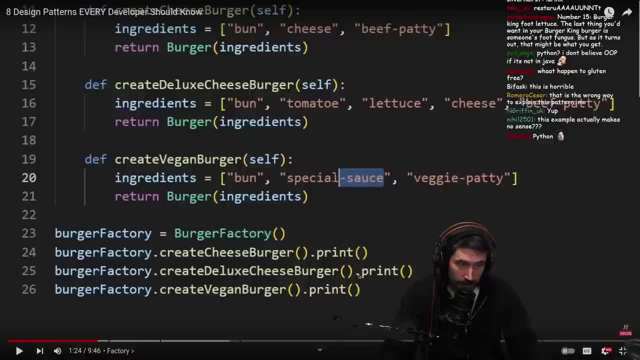 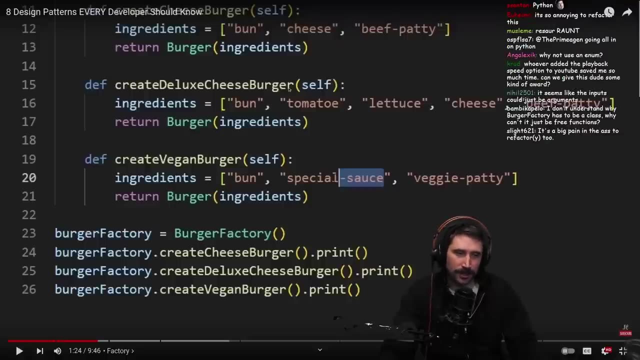 They all have the word print. Yeah, this example makes no sense, I agree with that, But the print thing at the end, this makes a lot of sense. Why not use an enum? I don't think this language-. I mean, at this point you should probably compose a burger. 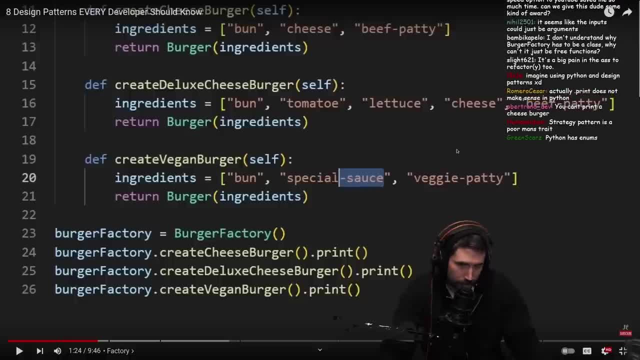 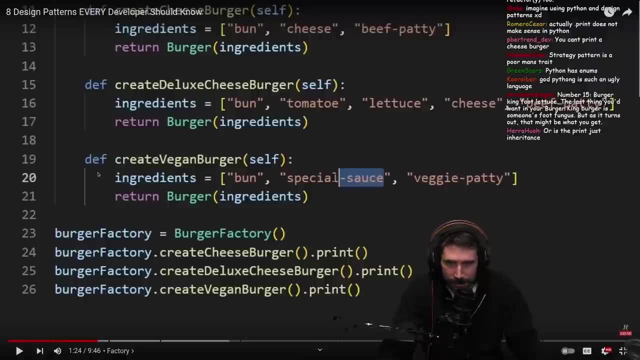 of its various topics- Toppings, Because you should be able to push a topping and make your own. Then you can have named ones. right, You should just have named ones. You don't have to create new instances. They should just be named hard-coded ones. 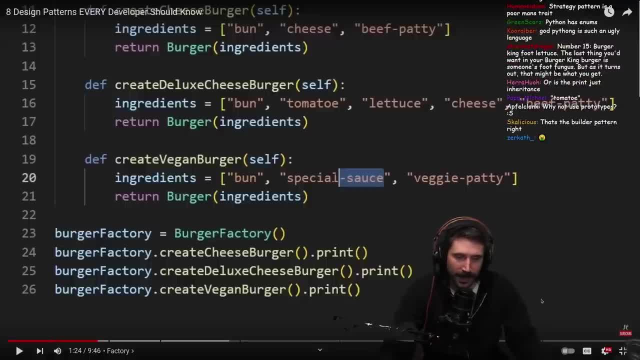 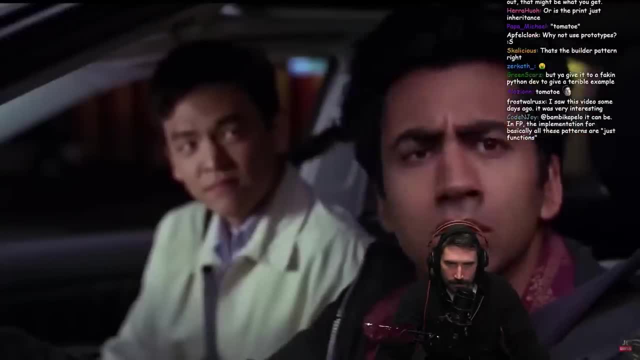 And then you can have your build your own one, right? Well, let's be real here, Okay, Anyways, You never know what's inside the special sauce. We have a secret ingredient: It's semen. Now, alternatively, if you want a little more control over how the sausage is made, you 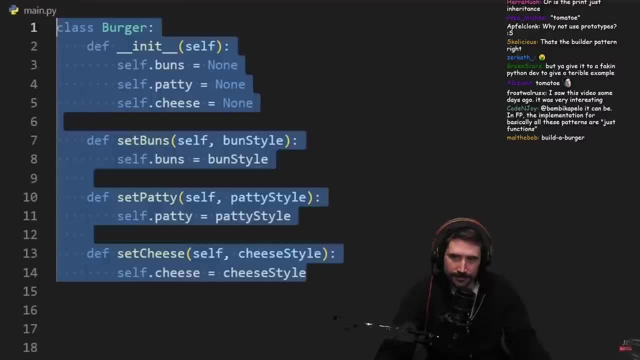 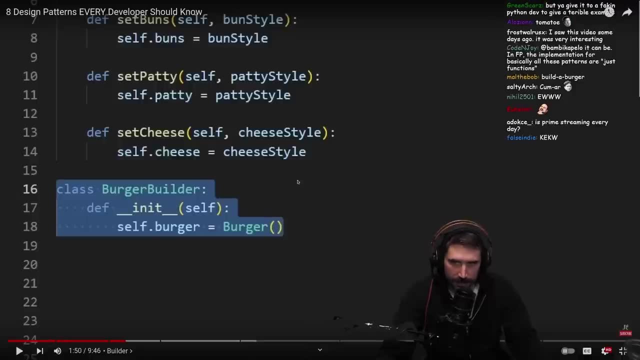 can go with the builder. The idea is that if we want to make a burger, we don't immediately have to pass in all the parameters. We can use a burger builder instead. We'll have an-. By the way, this is the better way to do things. 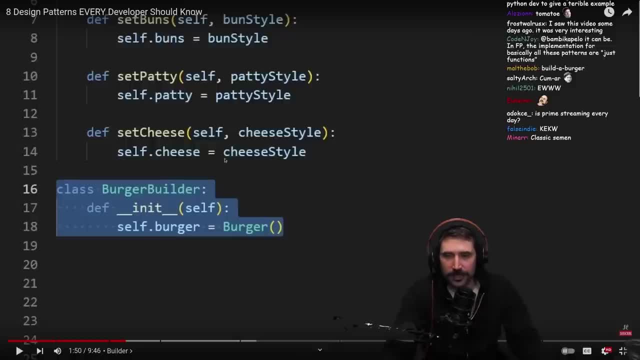 Sort of This whole- It is better. It is- And generally you should always use a builder pattern. Rust has a builder pattern. This is- This is a real- This is a real- This is a real good. This is always usually much better. 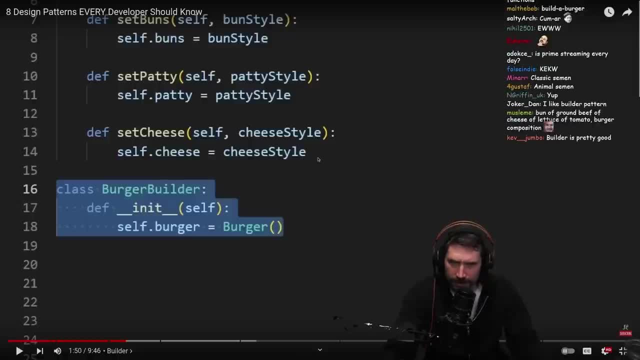 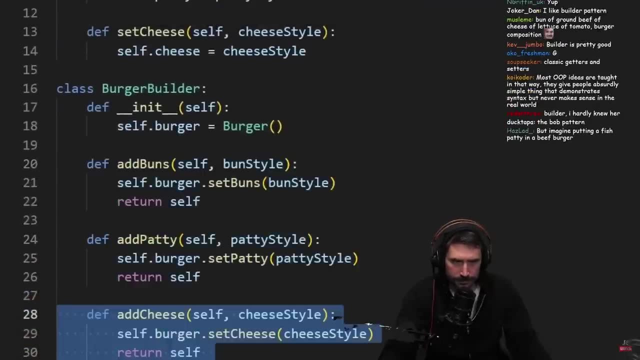 This whole like not returning yourself, though This is kind of freaking me out. Like you should return yourself, Return yourself, Return yourself. Individual method for adding each ingredient, whether it's a bun, patty or cheese. each. 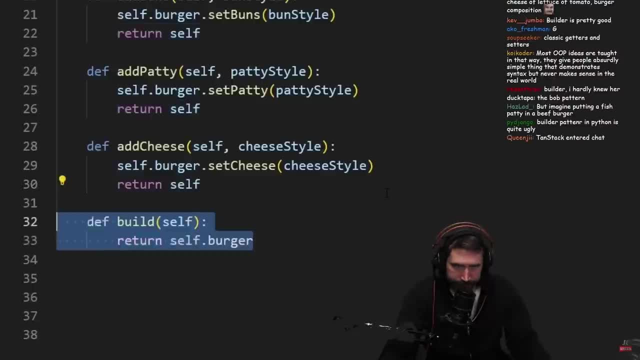 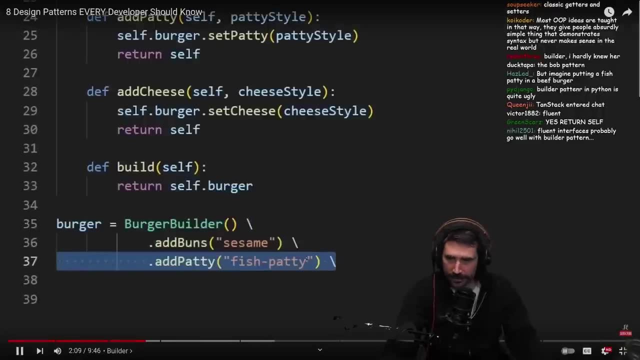 one will return a reference to the builder And finally we'll have a build method which will return the final product. Then we can instantiate a burger builder, add the buns that we want, the patty that we want and the cheese that we want, and we can change- 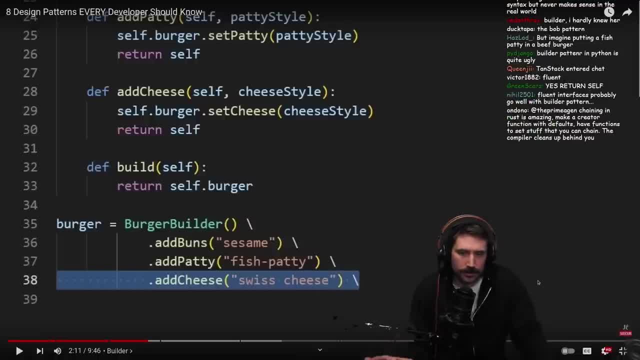 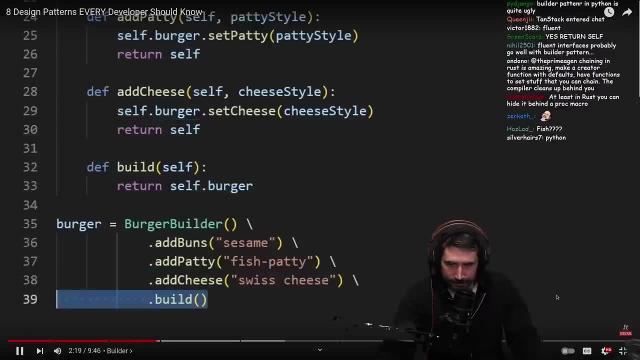 What is this Bash? What are we writing Bash right now? Change these methods because, remember, each one will return a reference to the builder. Finally, we can build it and we have the exact burger that we want. I've used this pattern a lot. 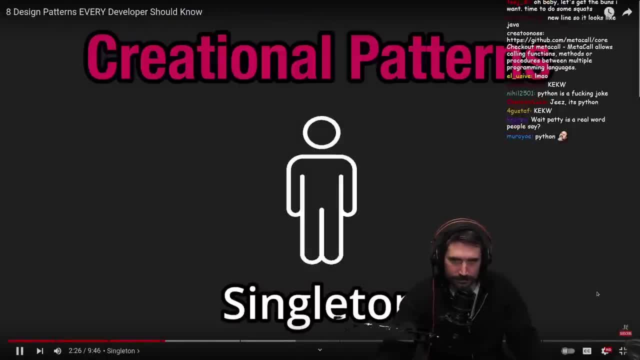 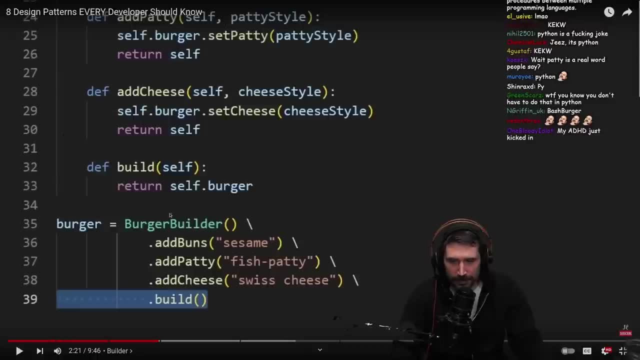 I've used this pattern a lot at Google with protocol buffers. Next we have the singleton pattern and I'm not- I did- You know he just lightly threw out using these with protobuffs Like that is a really great thing. 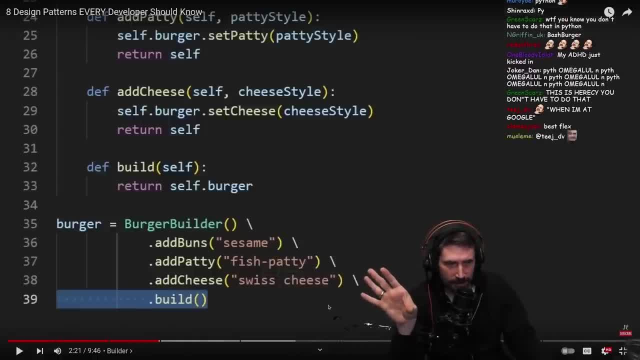 Protobuffs are amazing and this is one of the reasons why they're so good. When I'm at Google, I know: just tosses out- Casually tosses out Google and protobuffs, It's a-. Niko is absolutely right. 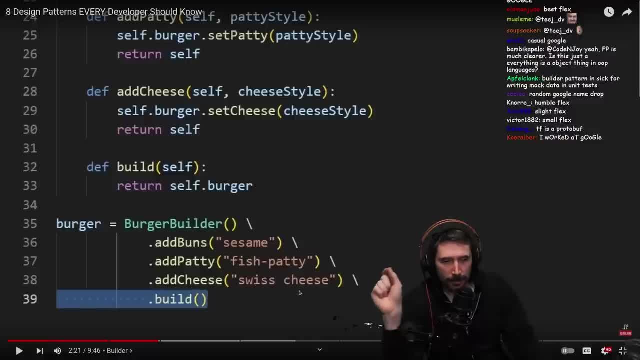 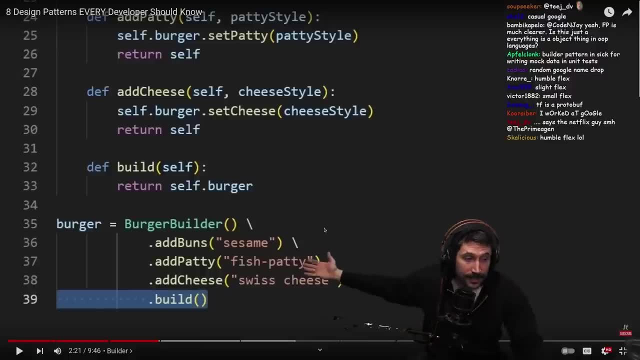 Like when you use- When you use proper builder patterns, which is just like something you see all the time. So this is like a good thing you can actually take Like: use this Honestly, use this today, says the Netflix guy. 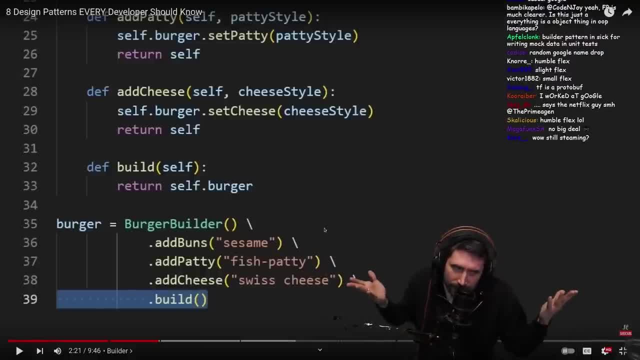 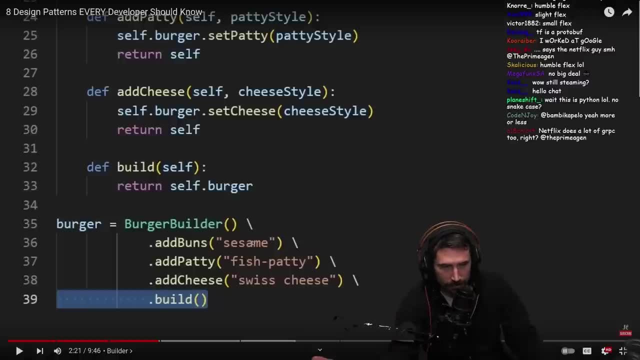 You know, when I'm designing my software at Netflix, I tend to use the builder pattern as well. You know what I mean. It's like this is actually a really good-. This is a very useful idea in general and it works in a lot of languages. 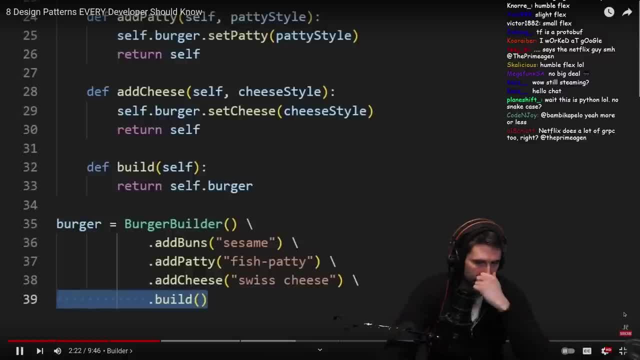 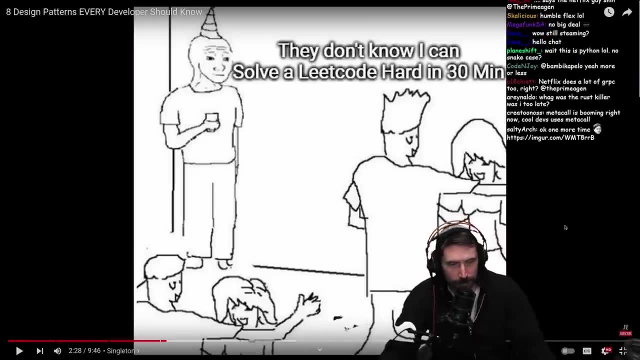 It's- Right, It's just good times. I've used this pattern a lot at Google with protocol buffers. Next we have the singleton pattern, and I'm not talking about- They actually renamed the singleton pattern, of course- to the arch user pattern. 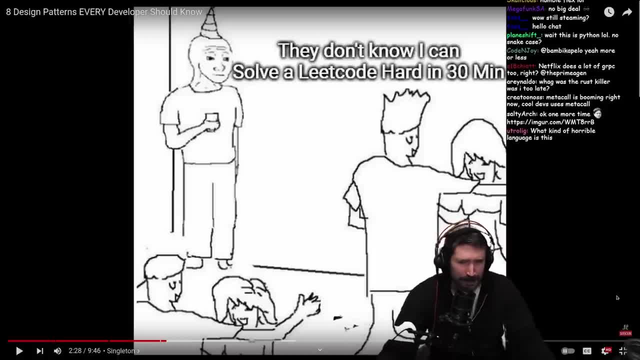 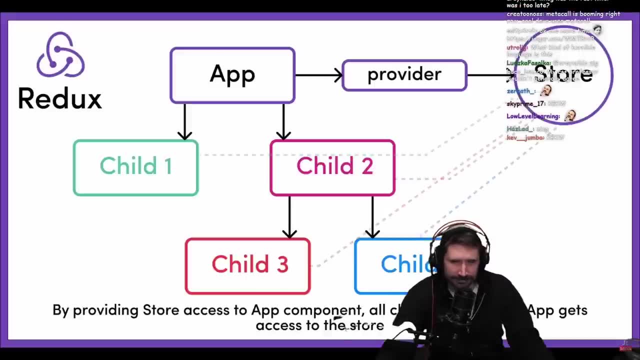 I mean you should probably- I don't know. You should probably keep up with the times. you know My dating life. A singleton is just a class that can only have a single instance of it. that's instantiated. It has many use cases. 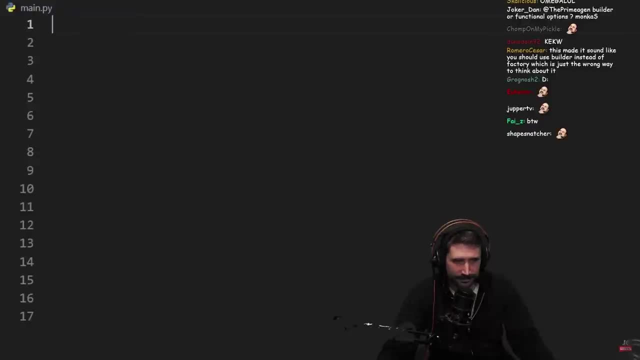 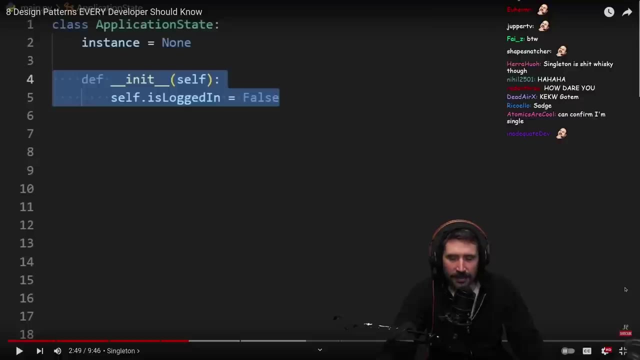 For example, maintaining a single copy of our application state. We would start by having a static instance variable. Let's say, in our app we want to know if a user is logged in or not, but we won't- I know that Python is considered like the worst language to do classes in. 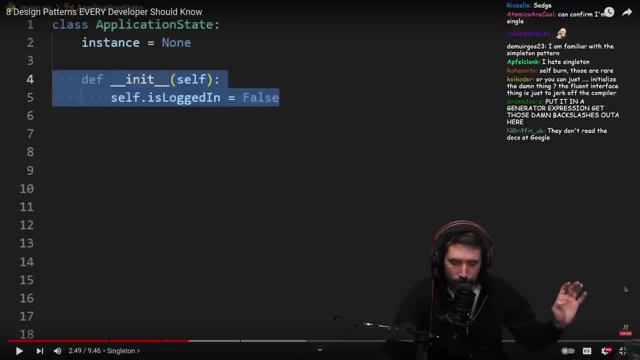 Just- Just be okay with it, right? We're looking for the pattern, Right? That's one cool thing That should make the pattern even cooler, in the sense that the pattern can exist in such a way that it can work in multiple different languages. 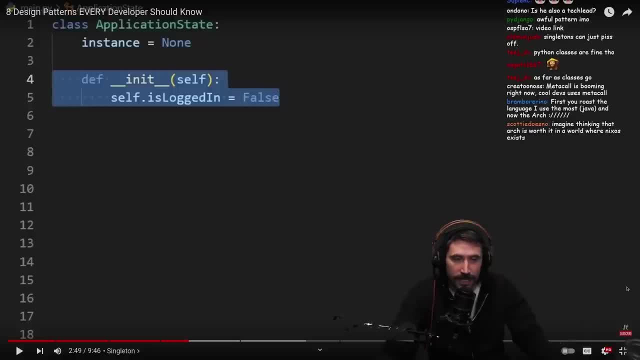 Right, That's good. That's a good thing, Because that's something that means that you can take it with you. The singleton pattern sucks until it's really awesome, Right? You know, I always come up with this stupid like database connection pool thing. 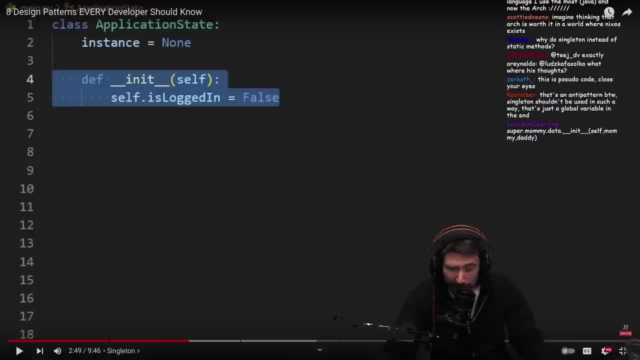 Sometimes you want it as a singleton, but then you're like: well, do you really want it as a singleton? Shouldn't your program just hold onto it? By the way, low-level learning: we did react to yours. Yours was great. 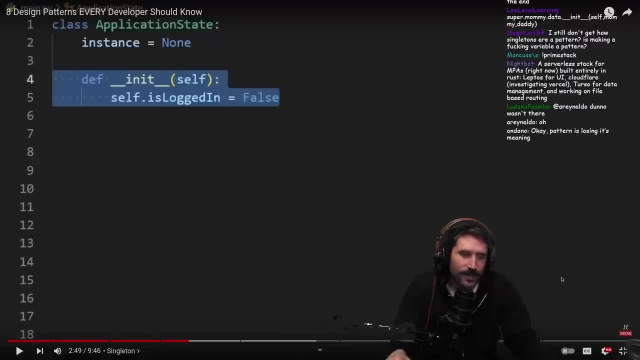 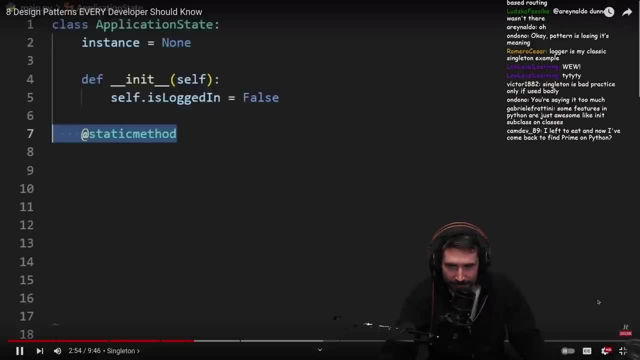 Your zig one. You know you always get into this one, you know. Don't use the constructor to actually instantiate the application state. We'll use a static method called get app-. Hey, low-level learning. can I do one more? react to one more of your contents. 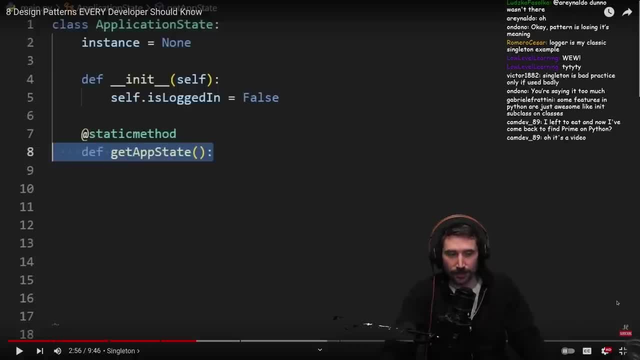 Can you pick your favorite one and send it to me? Yeah, yeah, yeah, yeah, yeah. We'll do one more after this Okay State, which will first check if there's already an existing instance of-. Can we pause it for a second? 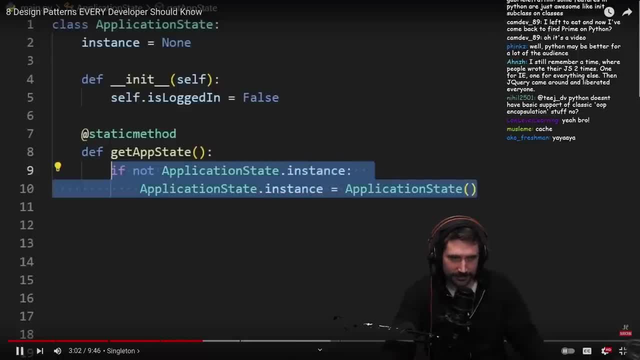 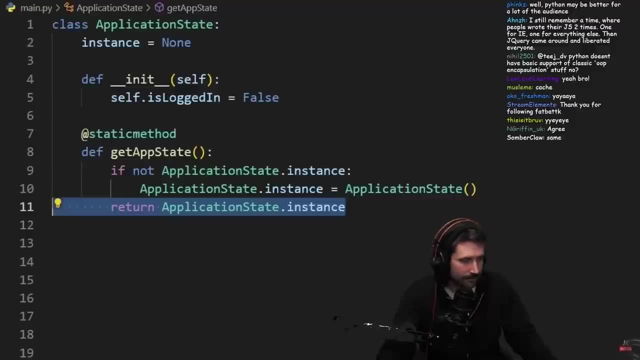 I hate decorators For application state. If not, we'll instantiate one. If there already is, though, we'll just return the existing instance. We'll never create more than one. So now, if we get our app state for the first time, the logged in value will initially be false. 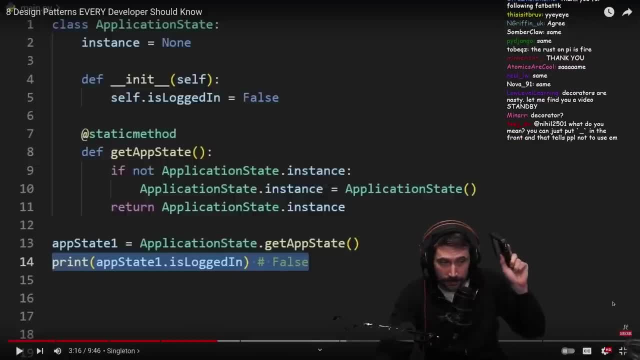 But if we- I mean to be fair, I did use a singleton pattern for this when I was writing the video driver and the audio driver. The thing was is that I also wrote the driver in such a way that behind the singleton was a strategy pattern. 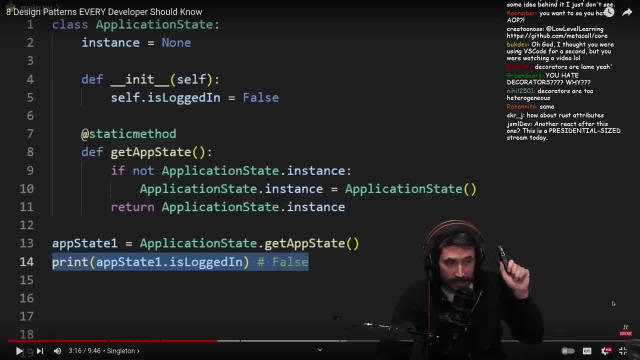 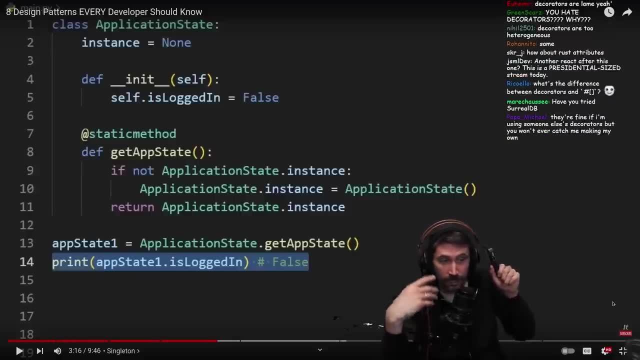 So it'd create a singleton strategy pattern. So that way I could write a sync player, something that doesn't actually go To anything, It just is like a software sync. It just swallows all the video and audio. So that way I could do like high performance testing right. 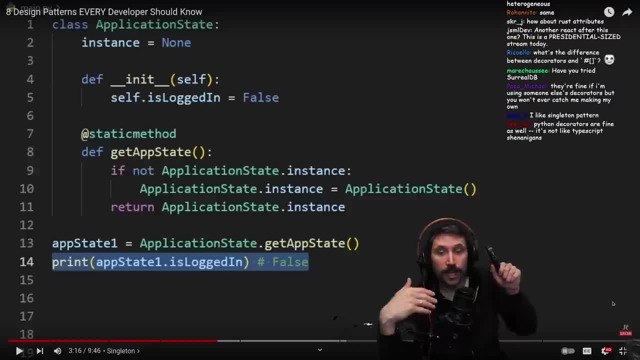 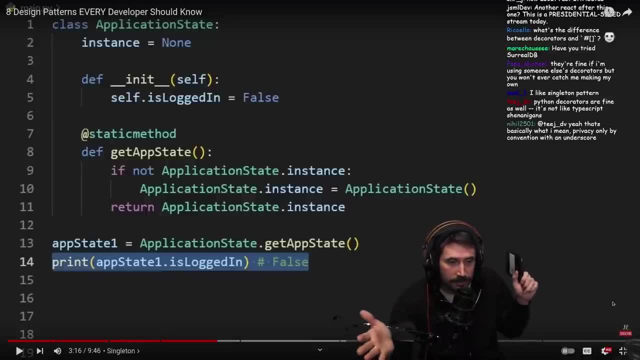 I could play two hours of video in five seconds, Or I had it really actually go out to the actual television, And so there is places where the singleton makes a lot of sense, And especially if you can mix in like a singleton with a strategy. 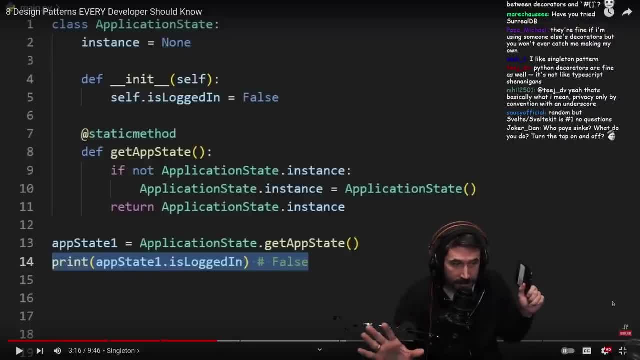 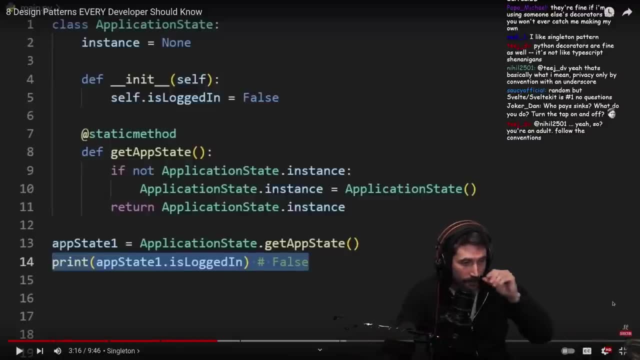 You can create ways to create your whole system such that it makes a lot of sense. So just saying, you know, I know the singleton gets a lot of uh Riff, raff, but there are a few places where it's it's super useful for me. 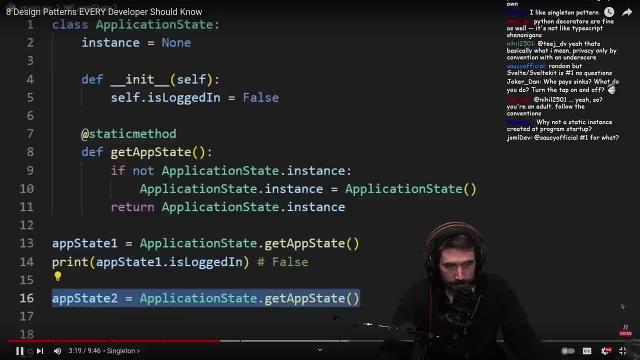 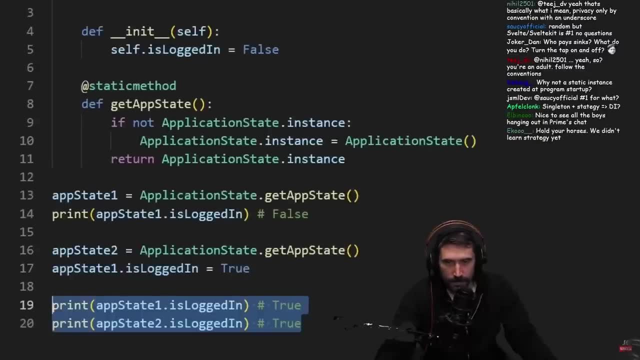 That was super useful. If we get the app state again, this will actually still be the first instance. So if we modify the first instance and then print the logged in value for both of them, they will both now be true. This pattern can be useful so that multiple components in your app will have. 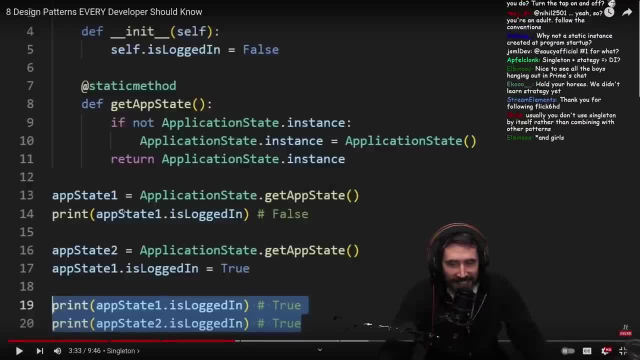 Also, this example is terrifying. I hate the idea. you know, modifying a static, a singleton, you know it just terrifies me. you know, like this right here, This thing terrifies me. I know it's not dude, it's crazy. 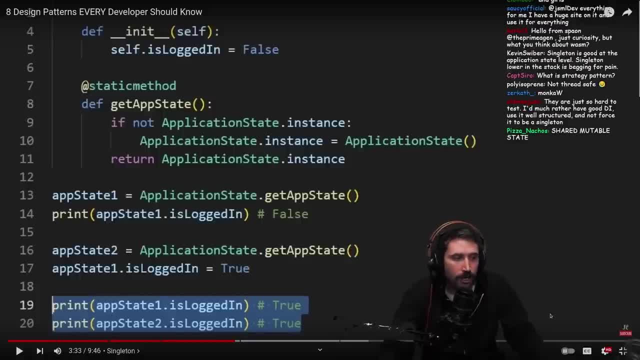 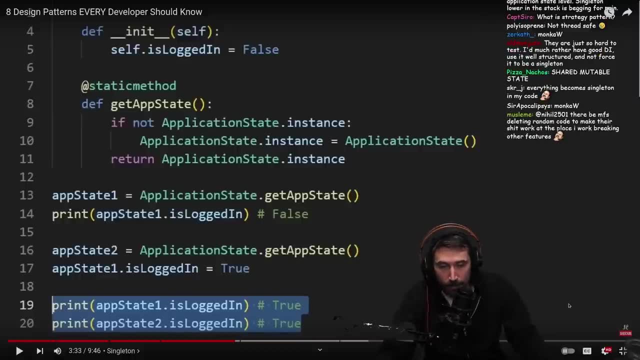 It's crazy. Uh, they're just so hard to test. They are so hard to test. I'm totally on your team with that Shared mutable state. It's shared mutable state is the the bane of all programming and the key to super awesome, amazing performance. 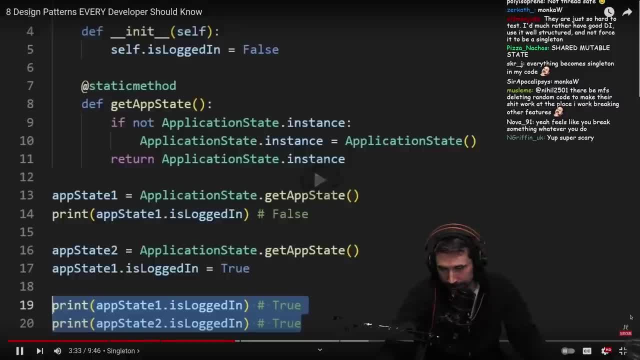 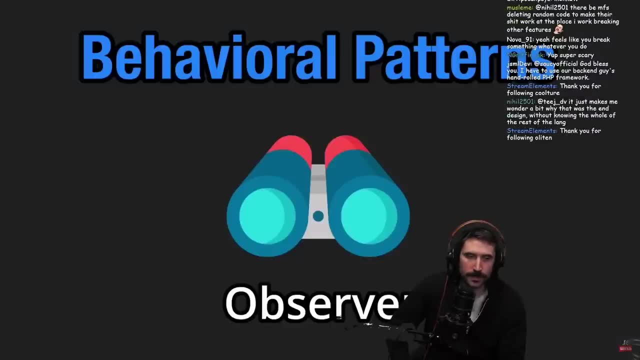 And it's the scariest thing in the universe. And so careful Have a shared source of truth, But how can all the components listen for updates in real time? Well, that's where the observer comes in: The observer's behavioral pattern. 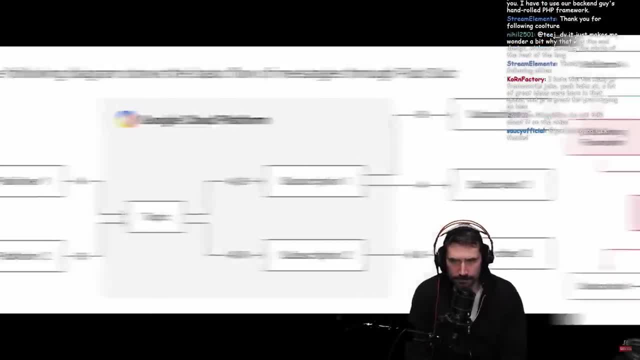 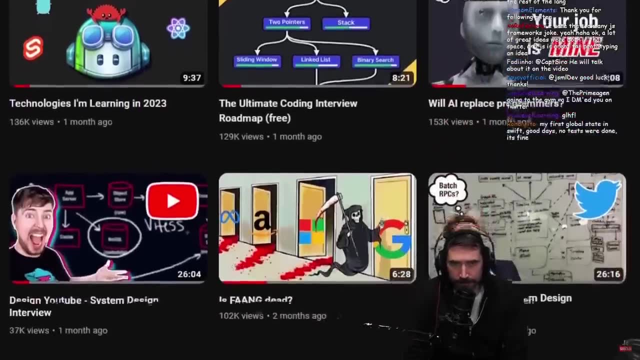 I prefer to call it the pub sub pattern. It's widely used beyond just object oriented programming, including in distributed systems. Let's take YouTube, For example. every time I upload a video, all of my subscribers get a notification, including you, because you're subscribed, right. 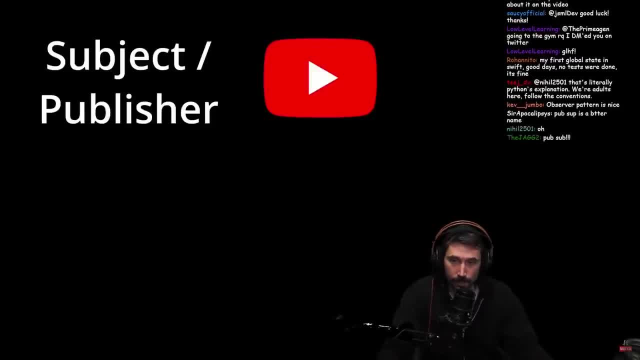 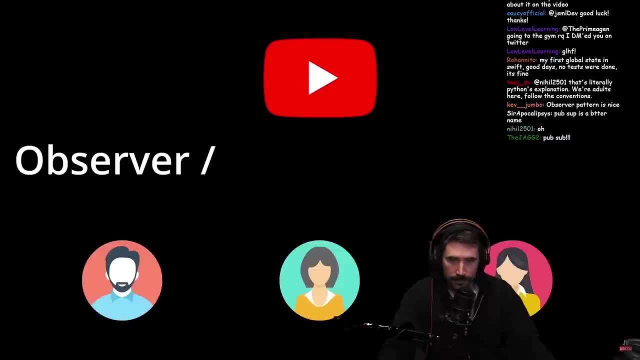 But in this case, the YouTube channel is the subject- AKA publisher- which will be the source of events such as a new video being uploaded. We might want multiple observers- AKA subscribers- to all be notified When these events happen in real time. 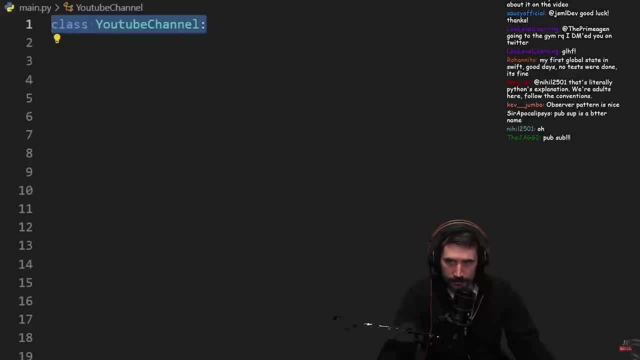 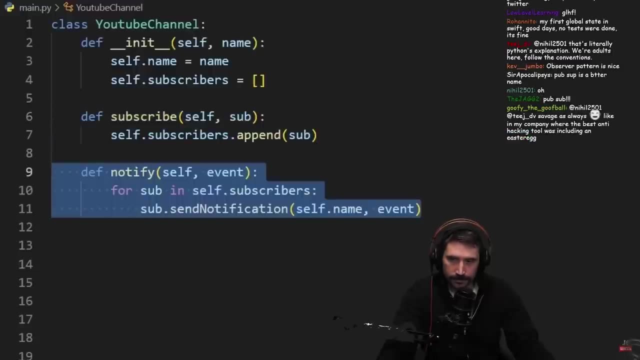 One way to implement this pattern is to have a YouTube channel class which maintains a list of its subscribers. When a new user subscribes, we add them to the list of subscribers. When an event occurs, we go through that list of subscribers and send the event data to each of them with a notification. 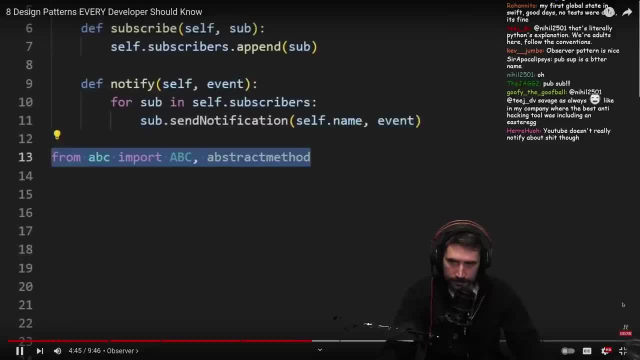 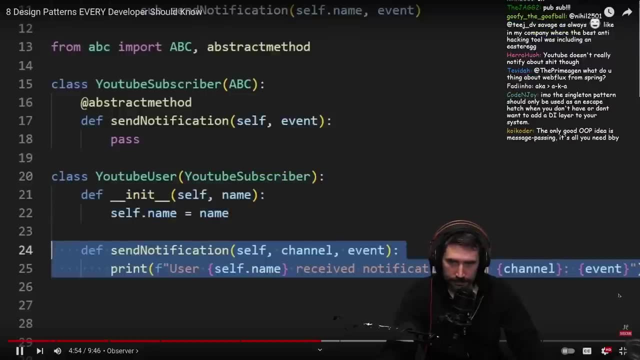 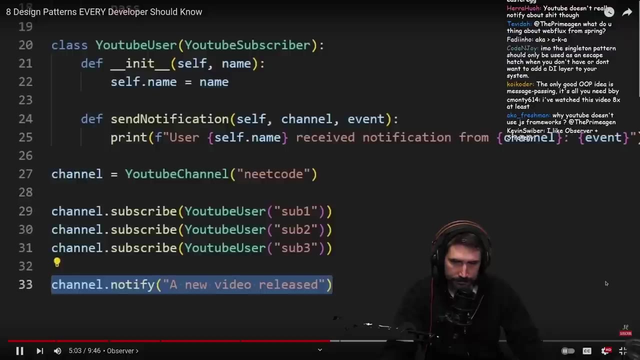 But we also have to define the subscriber interface, which you can do with an abstract class or an interface. Different subscribers might implement this interface differently, but for a YouTube user, let's say that we just want to print the notification So we can create a YouTube channel, add a few subscribers and we only have to call notify once and all of the subscribers will receive the notification. 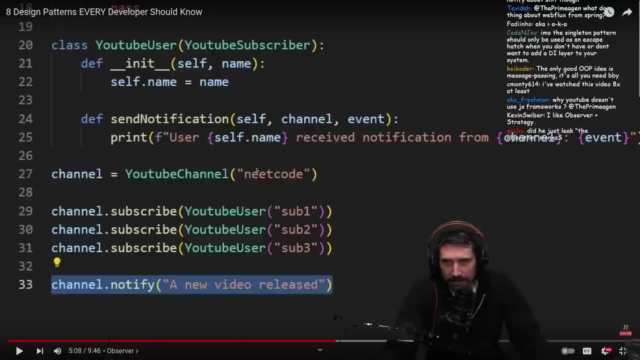 This is also. this is good. I mean, I mean observer pattern, It's, it's real time. Uh, we use this a bunch, I, you know again the Python. I think there's like an instant distaste for, for this, the idea of message passing. 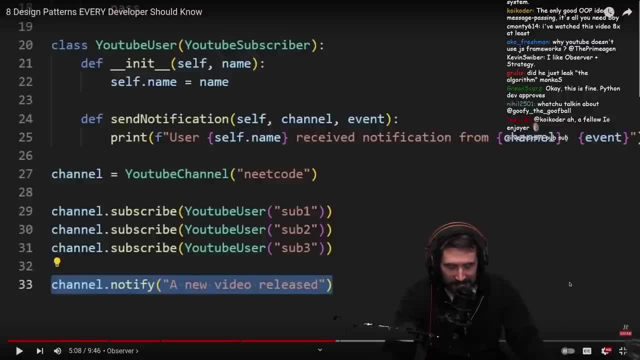 I know, Oh, my goodness, Don't shut up. TJ, TJ. Next thing you're going to do is you're going to start talking about objective C, So extensible enough. Yeah, I'm going to say that a subscriber could be subscribed to multiple channels. 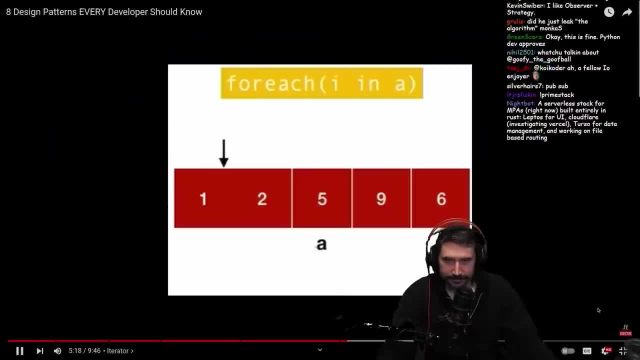 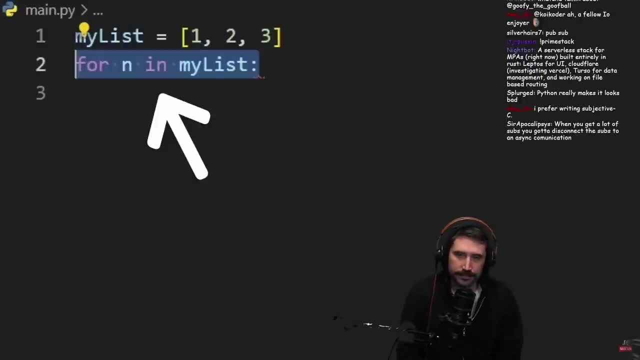 An iterator is a pretty simple pattern. It defines how the values in an object can be iterated through. in Python, Just defining an array and then iterating through it with the in keyword uses the built-in list iterator. This way we don't even have to index the array. 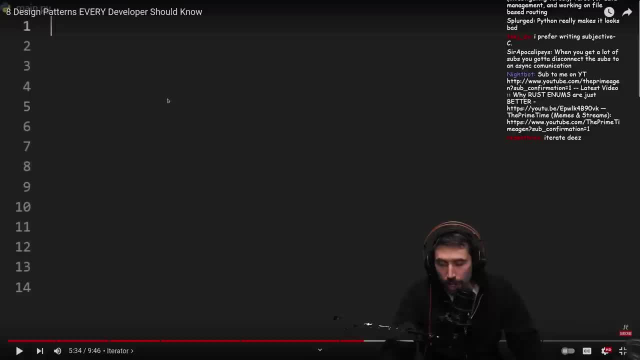 Now for more complex objects. Iterators was a good one. In fact, you should know an iterator pattern. Uh, one of my first interviews with Google, like 10 years ago when I had to fill it out on Google docs- I actually did the Google interview at my job. 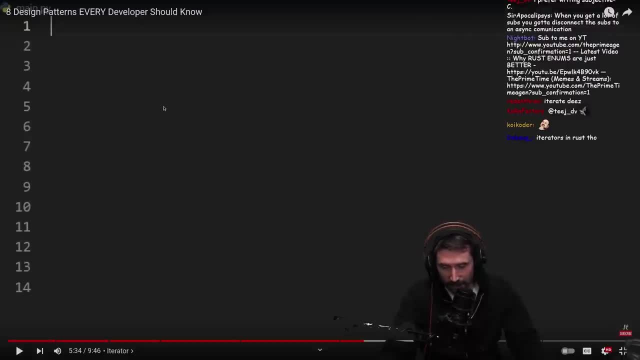 at my job when i was writing c for the government, for robots, and at google, by the way, i got rejected, by the way. they didn't like me, by the way, but part of that interview was to write an iterator right and so and so, knowing iterators, iterators are super useful. they're, they're, it's a, it's a. 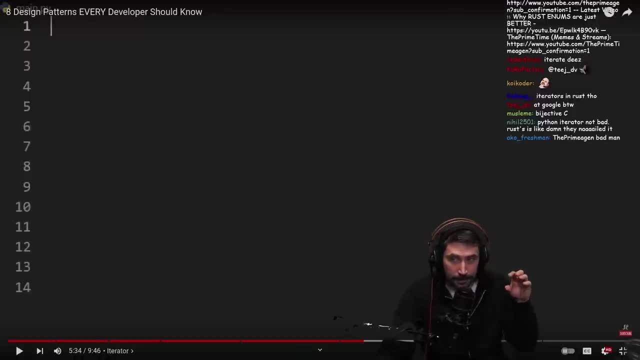 great pattern and i've used iterators as ways to solve problems at netflix, by the way. by the way, i- i work at netflix, by the way, uh, and so it's like it's really really good. yeah, yeah, netflix, or google, did reject me twice and then they offered me a salary lower than the one i have at netflix. 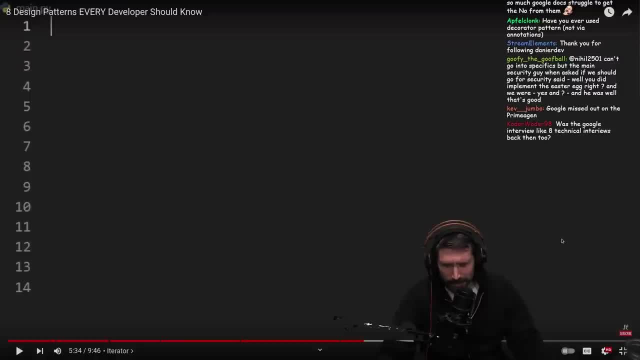 and tried to convince me that it's a starting point. and i said, of course it's a starting point. any point you give me is a starting point. what you're saying is an objective truth for an objectively bad offer. so try again. it's like binary search trees or linked lists. we can. 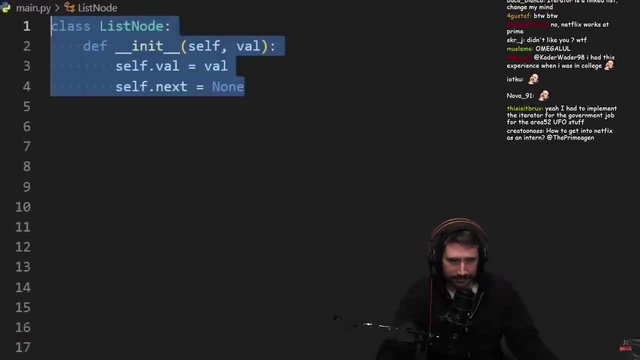 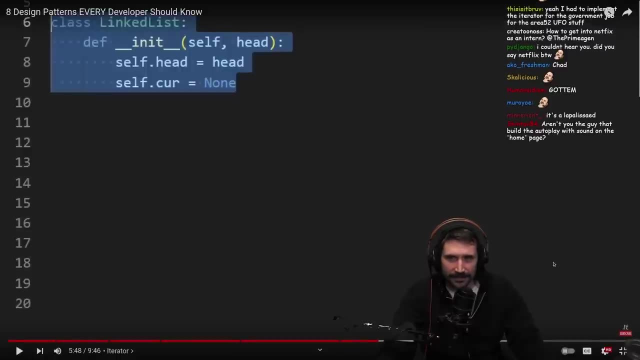 define our own. we can take a list node which just has a value and a next pointer, and then a linked list which has a head pointer and a current pointer. we can first define the weird passing in head as the first node. uh, you know, just saying, aren't you the guy that? 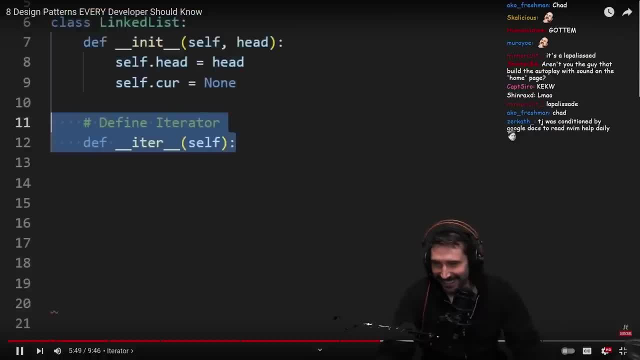 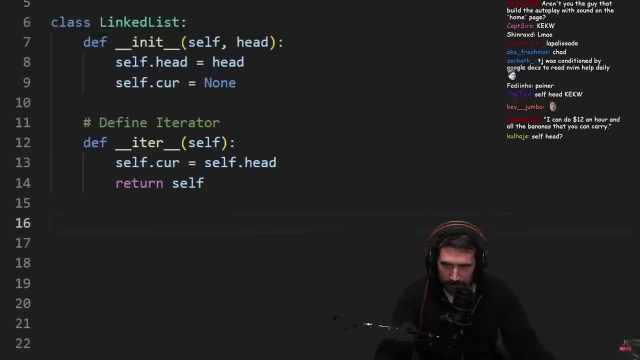 built the autoplay sound on the home page. i am iterator with the iter function, which will just set the current pointer to the head and then return a reference to the linked list to get the next value. in the sequence we define the next function. if our current pointer is non-null, we can. 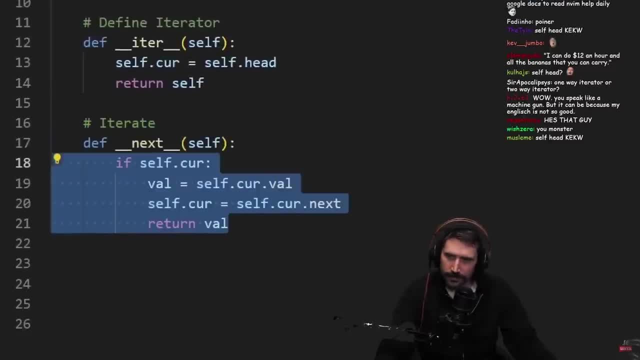 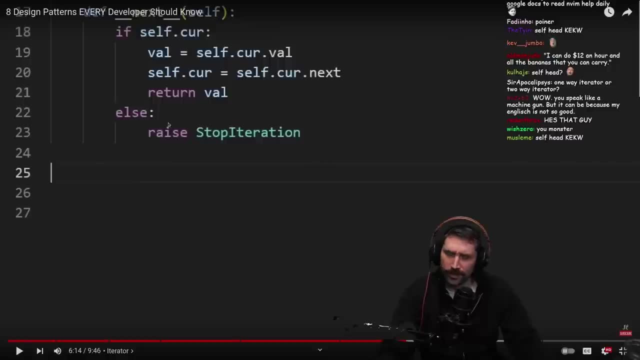 get the value and then return it and also shift the current pointer. but if we reach the end of the linked list, we can send a signal that we're going to stop iterating. to test it out, we can just initialize. that's weird, oh yeah, because they don't have options, do they? oh yeah, 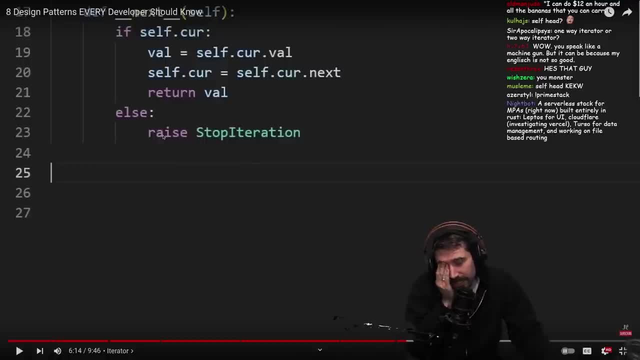 so russ solves this differently. you know, i don't. i mean this just seems like why do you? why you have to throw an error to stop iterating, just i mean it seems weird. right, can we agree that it's a little? it's just a little weird. you know, it's a little weird. i'm just saying it's a little weird, okay. 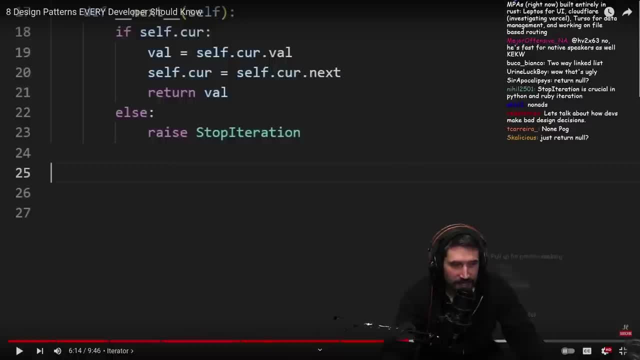 stop. iterating is a crucial in python. yeah, i know, but it's still. it's weird. how do i get into netflix as a software and- darn um be amazing list and iterate through it with the end keyword? this is a much more simple interface than having to actually update pointers. 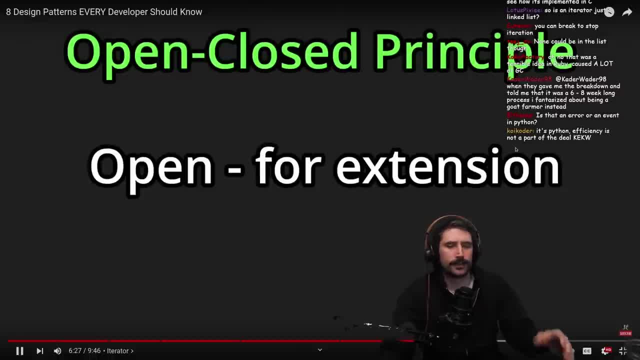 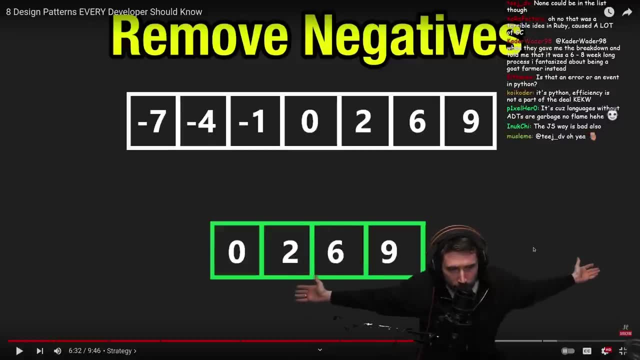 ourselves. now, if you want to modify or extend the behavior of a class without directly changing it, you can go with the strategy pattern, for example, we can always, just always use the strategy pattern, okay, just just. everything's a strategy pattern, that's all. strategy pattern is just fancy talk. 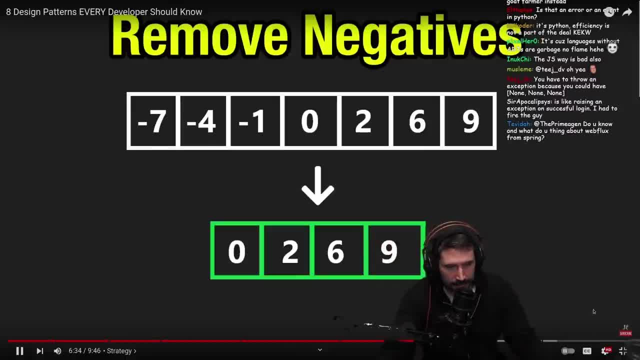 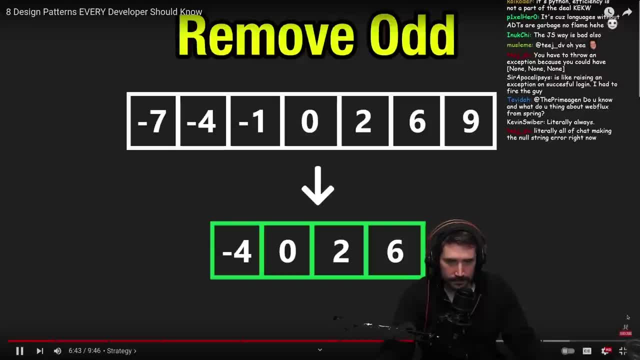 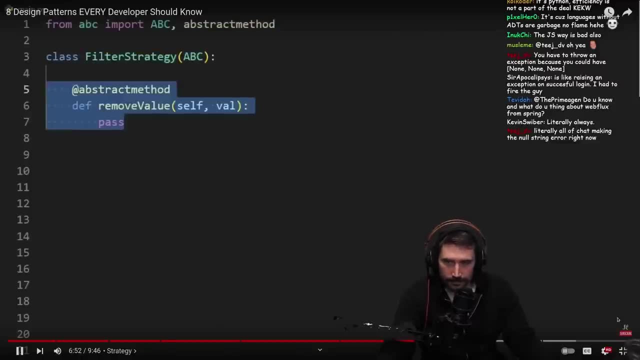 for use. an interface, you dummy. you can filter an array by removing positive values, or we could filter it by removing all odd values. these are two strategies, but maybe in the future we want to add more and we want to follow the open- closed principle. well, we can define a filter strategy, create an implementation. 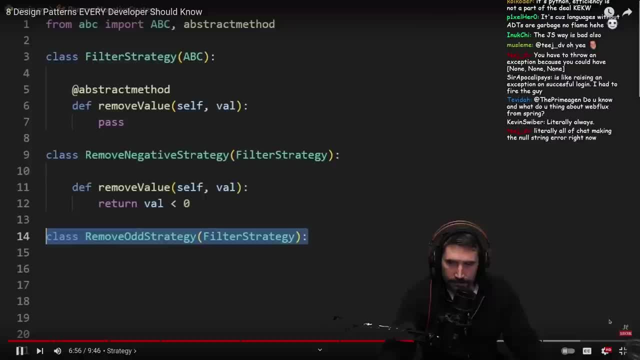 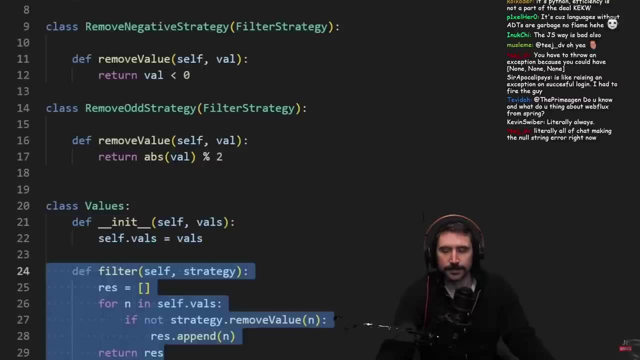 which will remove all negative values and an implementation which will remove all odd values, and then at runtime, we can pass this strategy into our values object and to test it out, all we have to do is pass in the strategy pattern and then we can filter it by removing all negative values. 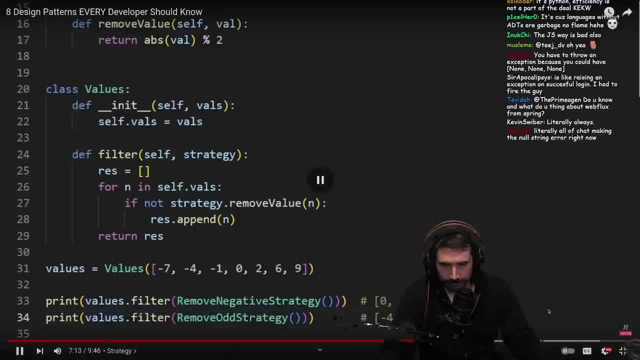 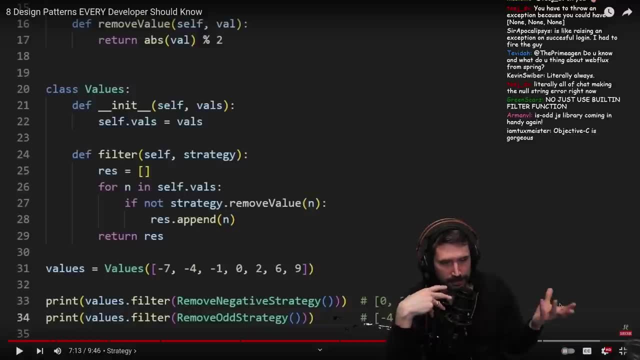 into our filter method and we'll get our desired result this way. we- i use this exact like. i literally use this exact same thing, so i had to create uh. so at netflix i'm doing this whole like performance audio video thing that i've been kind of talking about, and when i'm building up some of 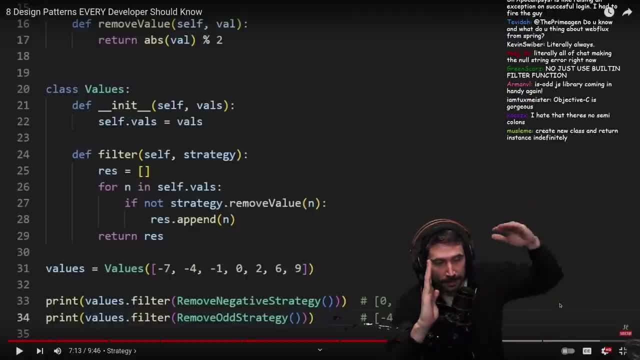 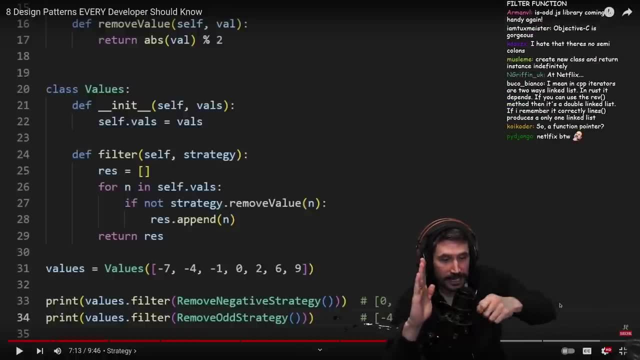 the data stuff. uh, there's some values that, as i build it up row by row, i need to use the previous value, uh, but there's other that i need to only use the values that happened within that specific time span. and so what i did is i created a filter method and i built it up, and i built it up and i 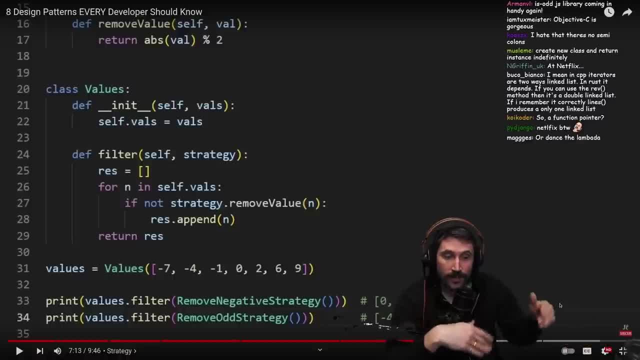 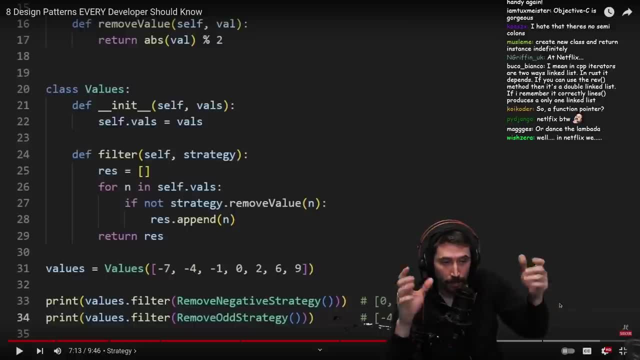 created an emitter right. so i have a continuous emitter, one that always emits the previous value, and then i have a counter emitter so that, as time passes, i only emit at that point what i saw at netflix. of course, by the way, i work at netflix, i don't know if you know that you can add additional. 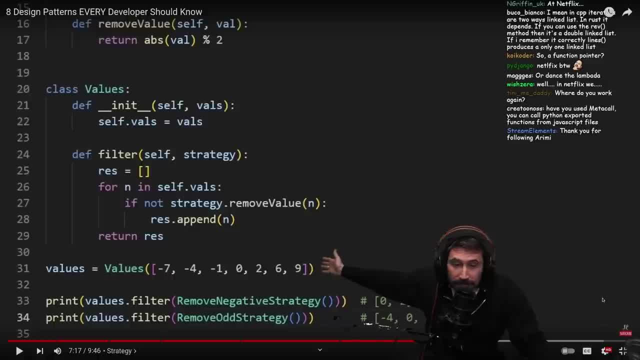 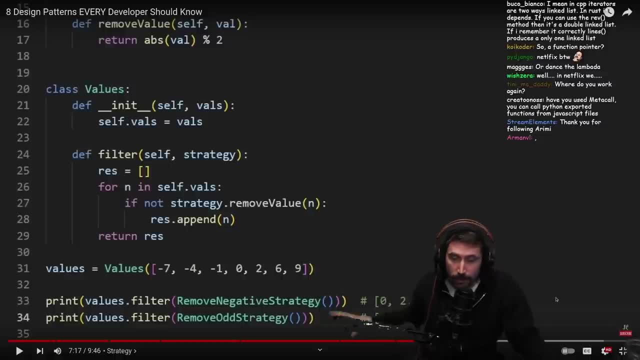 strategies without modifying. you don't even have to, you don't even have to like oop to love strategy pattern. strategy pattern is it's just make the thing into an interface and do the logic below the interface program at an interface level. that's all. strategy pattern is programming. 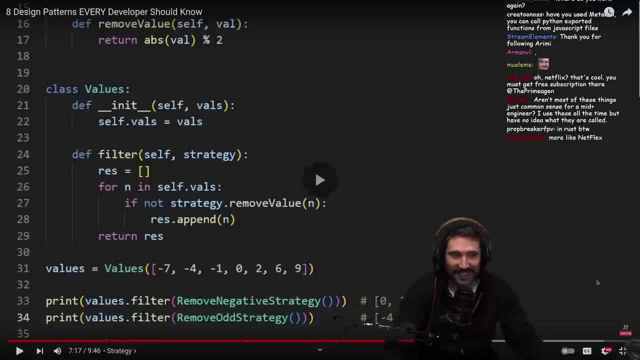 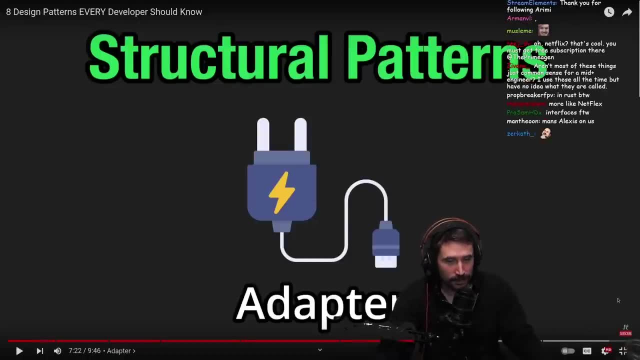 at an interface level. oh, netflix, you must get a free subscription shut up. we don't talk about our values class. next we have the adapter, our first structure adapter pattern, what i like to recall, the lose your hair slowly pattern rule pattern. it's analogous to the real world where 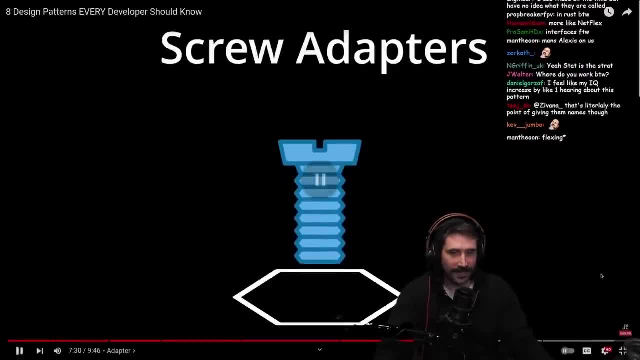 we have a screw that's too small to fit into a hole. so we've all, we've all felt this problem. okay, you know a lot of a lot of us. you know we're just trying to- uh, you know we're just trying to live our life. you know it's not my fault. 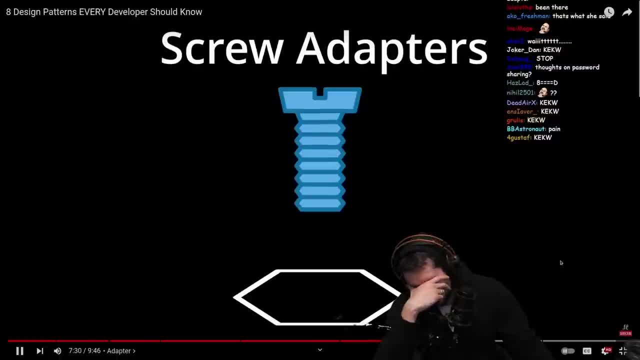 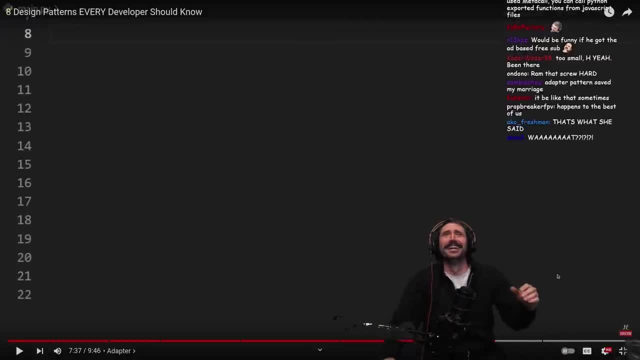 so instead we use an adapter which makes the screw compatible with the hole, or maybe an example: he just passed out the sexy sax man at the end. okay, well, i'm happy that. uh, i'm glad, i mean i'm very happy- that he leaned into that one. that was good. no one can be upset about that. 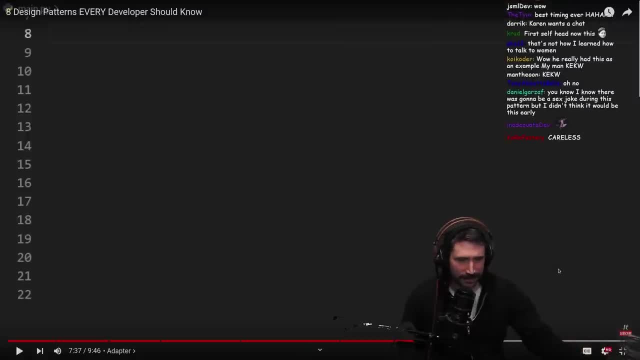 oh, that's a lot of water. no one can be upset about that. all right, keep peeing. i know i can't believe that, can't believe there'd be a sexy time joke here. well, that you're more familiar with. we have a usb cable and a usb port. we can plug in the usb. 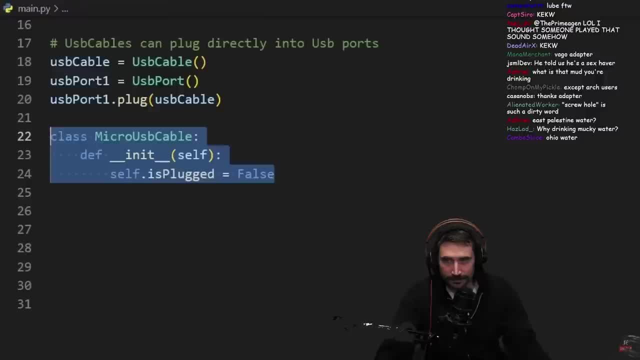 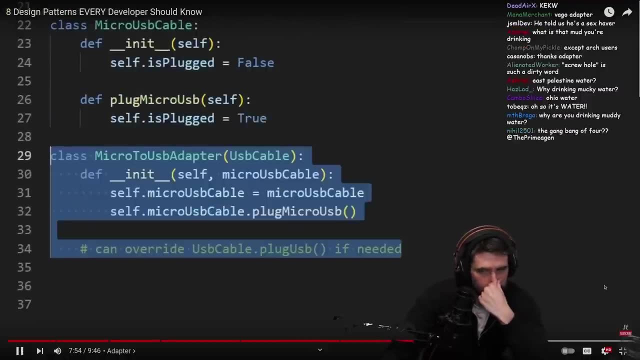 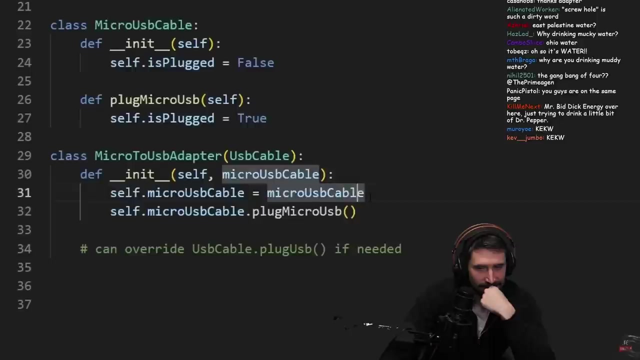 cable which will directly fit into the port, but instead, if we have a micro usb cable, it's not again okay, just because compatible. so instead we need a micro to usb adapter which extends from the usb class but is composed of a micro usb cable which will be plugged into the port and 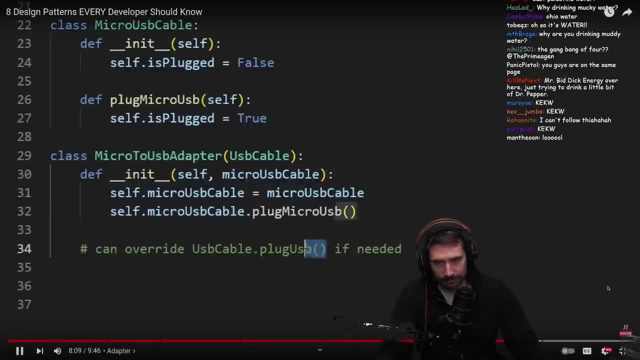 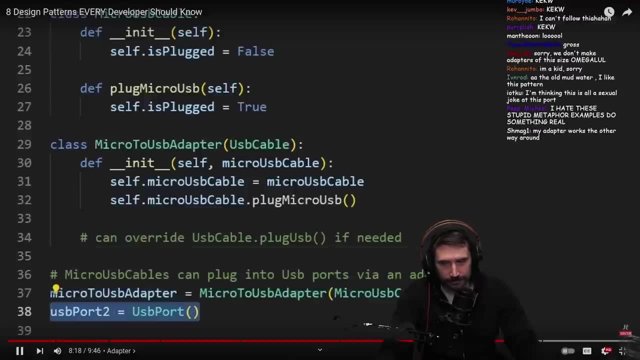 into the adapter. we can override the plug usb method from our parent class if needed, but it's not in this case- and then we can plug our micro usb cable into the adapter and then plug it into the port and it works just like a ray. this is pretty much. this is just pretty much the strategy. 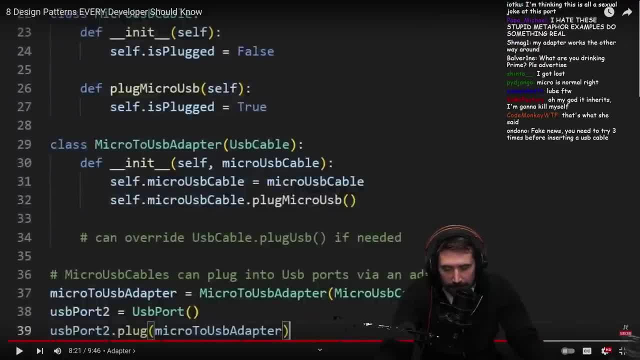 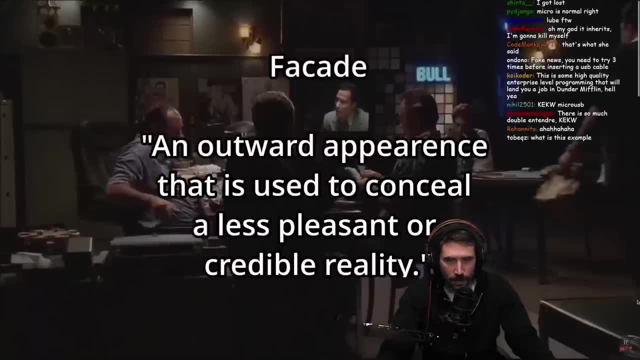 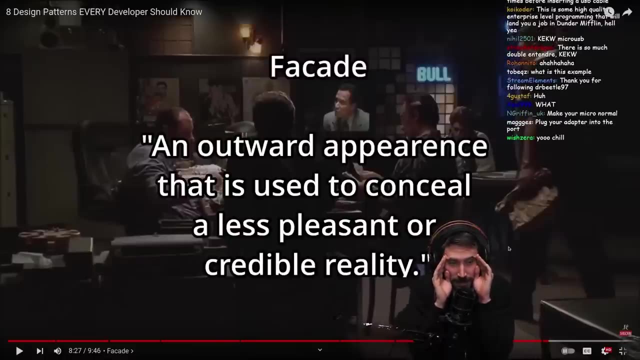 pattern again right, adapter pattern is just the application of a strategy. pattern thought is: is that regular usb cable? and our last pattern is the facade, according to the dictionary. so facade pattern- um, the facade pattern is actually okay. so remember that whole like types definition argument that we 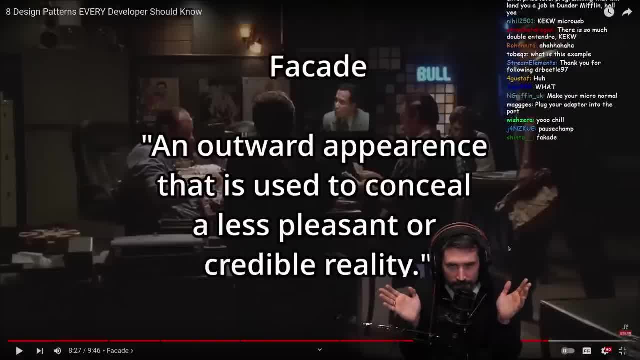 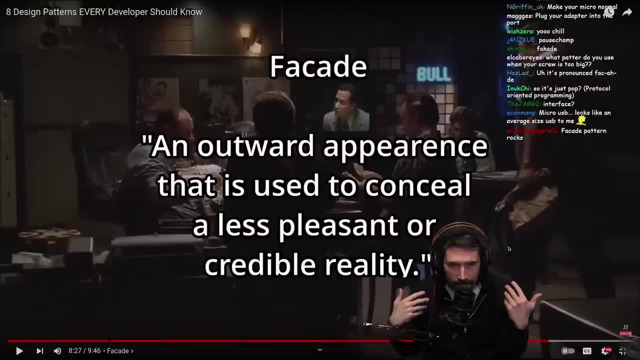 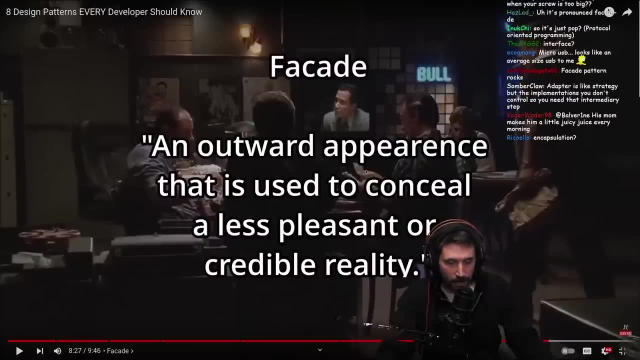 went over the whole return types and all that in theo's video video. one of the reasons why i love return types is that you can actually facade it, and this is really important. it's not facade, it's not facade, or however you're saying it's it's facade, uh, and so i actually like the facade. 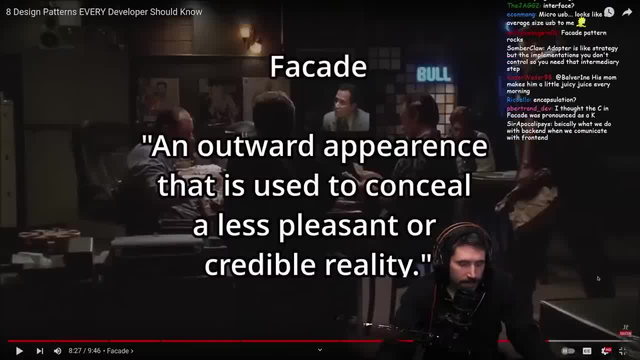 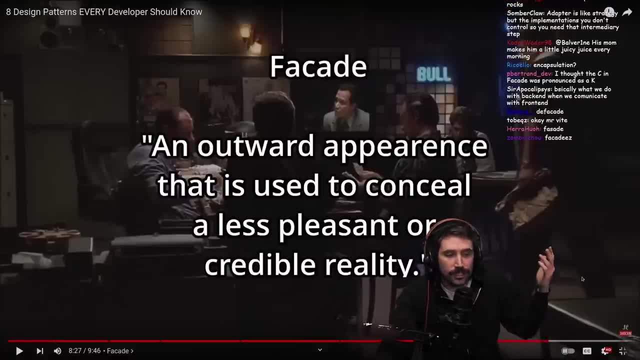 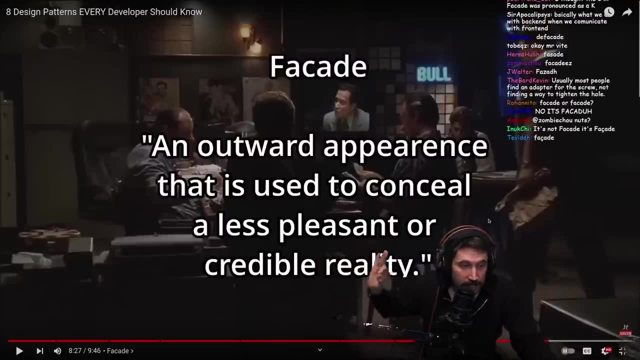 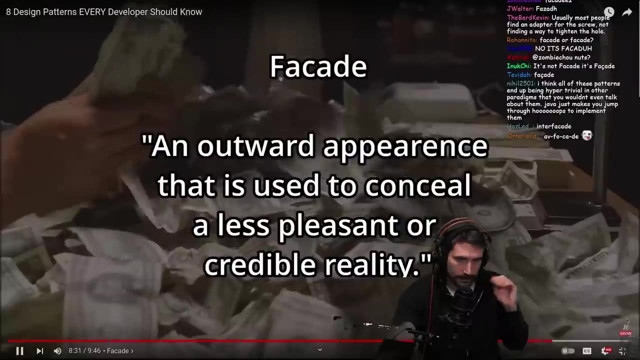 pattern facade. facade is just encapsulation. facade is just like a fancy ass word for simple, simple right, it's interface. again, it always just comes down to interfaces. this is just for facade, these nuts. it's just simply make an interface and not all interfaces need to be equal. okay, a facade is an outward appearance that is maintained to. 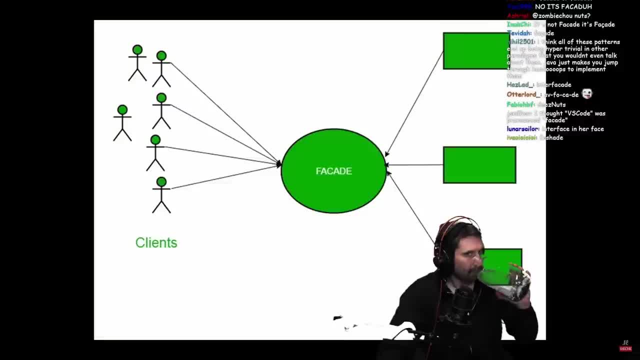 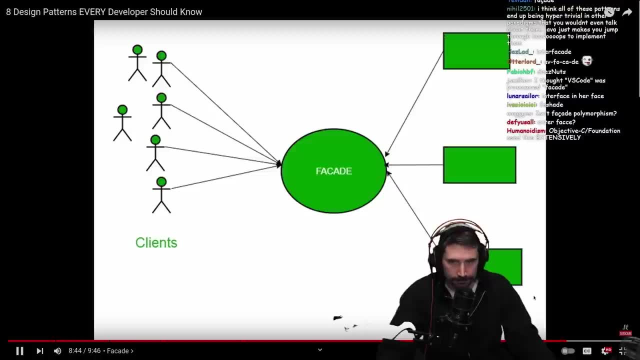 conceal a less pleasant or credible reality in the programming world. the outward appearance is the class or interface we interact with as programmers, and the less pleasant reality is, hopefully, the complexity that is hidden from us. so a facade is simply a wrapper class that can be used to. 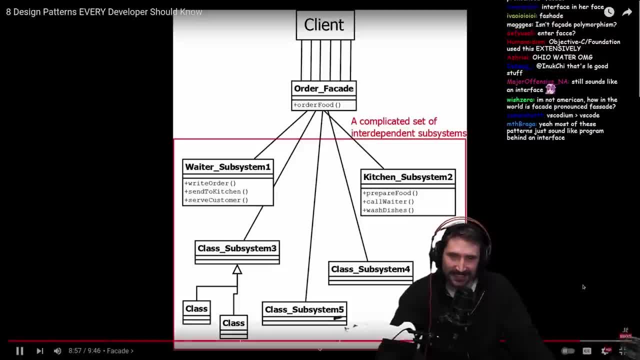 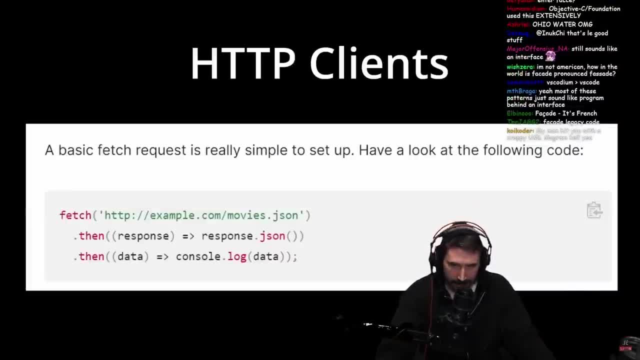 abstract lower level details that we don't want to have to worry about. i'm surprised it even qualifies as a design pattern, but some common examples might include http clients that abstract away low level network. this is perfect. this is a perfect example. you know that, like again, i, the 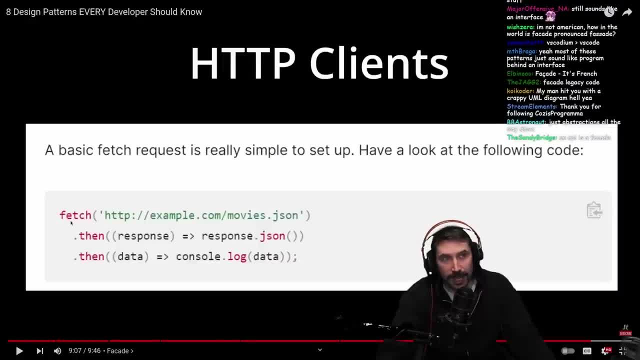 problem about the facade pattern is it's not necessarily a pattern as much as it is just good programming technique, because- because the thing is is that you can't really the. the thing about like, the, the strategy pattern, is that there's like, there's a, there is an inherent thing you can apply. 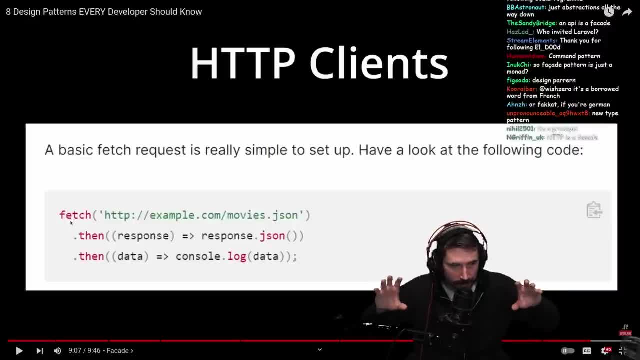 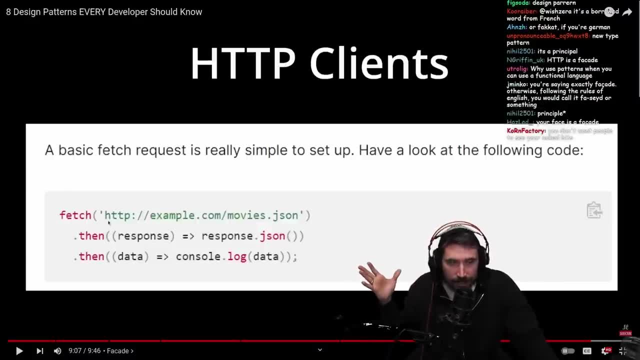 it to. you can inherently apply the observer pattern, you can inherently apply the singleton pattern. this one you can't just apply because there's no actual application. it's just like you take a bunch of stuff and you make it into a method for doing a thing. everything's a facade. everything's a facade, exactly. 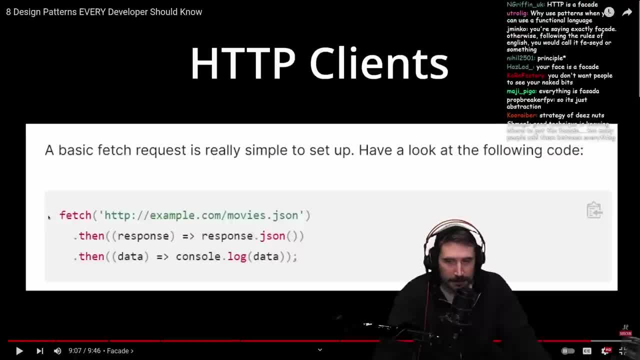 and so that's like part of the. the problem with this pattern is that there's no concrete application of it. you don't know, a good programmer uses it, a bad programmer uses it. a good programmer just uses it better than a bad programmer uses it. a facade pattern doesn't even have to be. 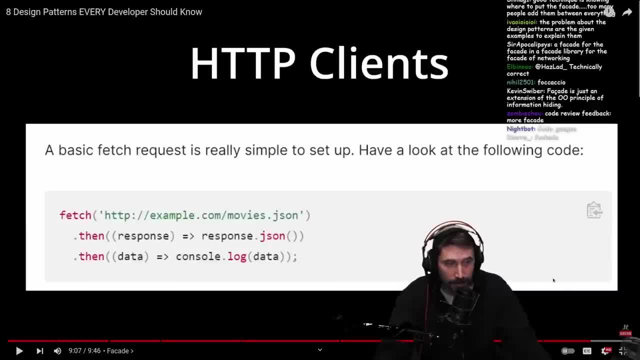 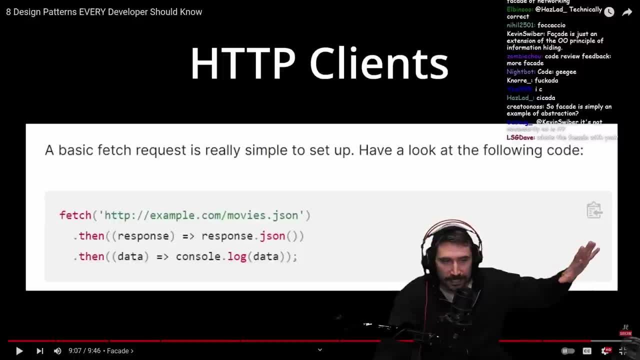 an extension of- oh, it's just an extension of- good programming. you can take any, anything that you can hide information from that best programming API. Ciao, Tom. so Kristandla for watching oure review job and you can have private implementation, implementation details and external ways.